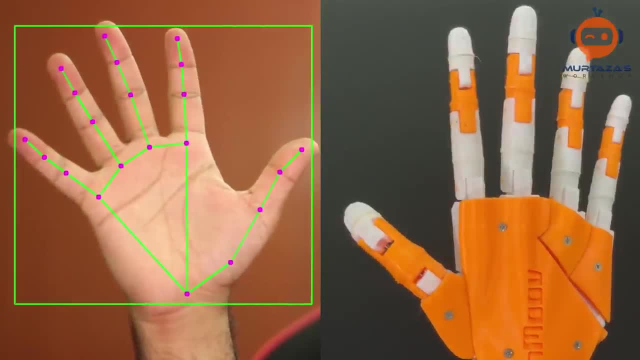 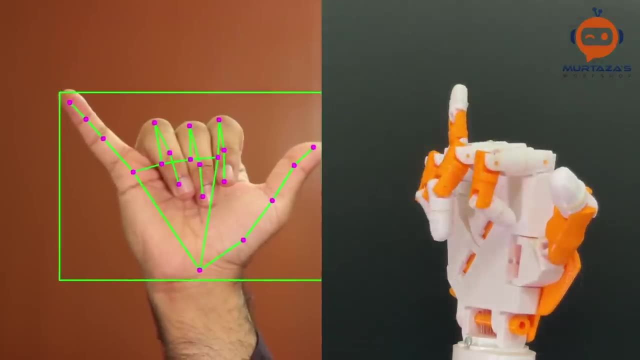 And all of this will be done with just 20 lines of python code. That's right. with our new CV zone library, building robotics and computer vision applications has become very convenient. If you would like to create real-world computer vision apps, do check out my premium course in. 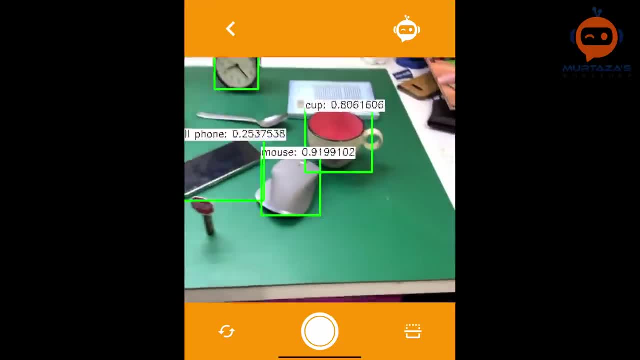 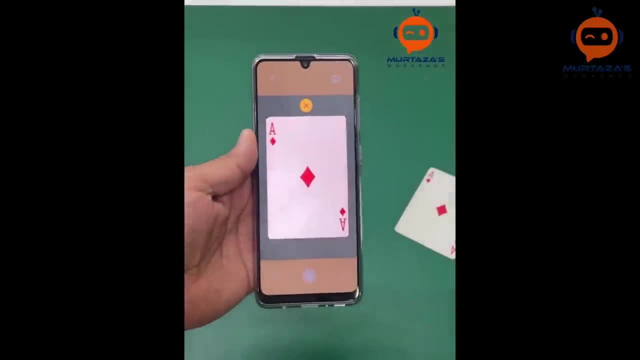 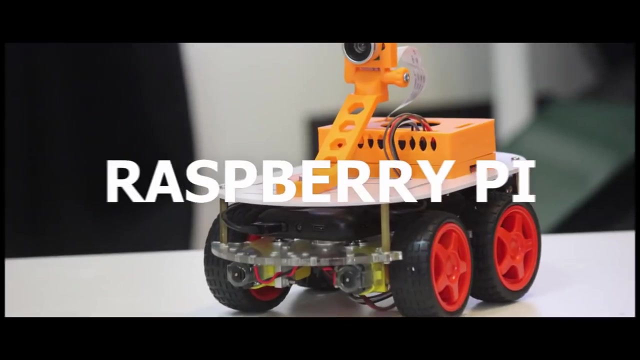 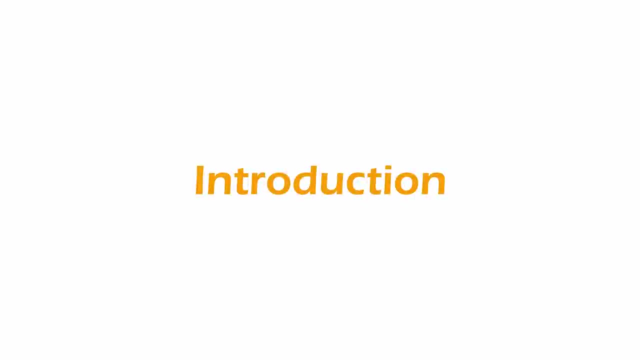 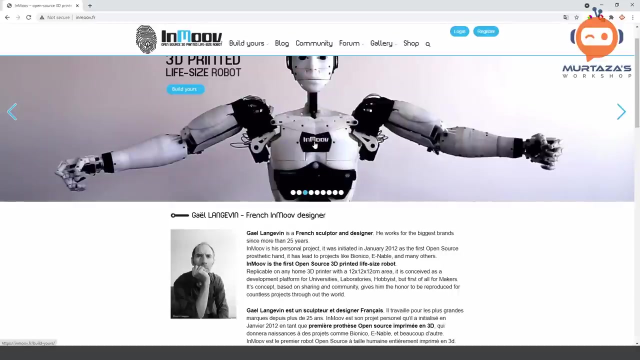 which we learn how to create apps such as object detection, augmented reality, document scanner and a lot more. The link is in the description below, So without further ado, let's get started. So the robot arm we are using today is by the InMove project. This is the InMove robot, As you. 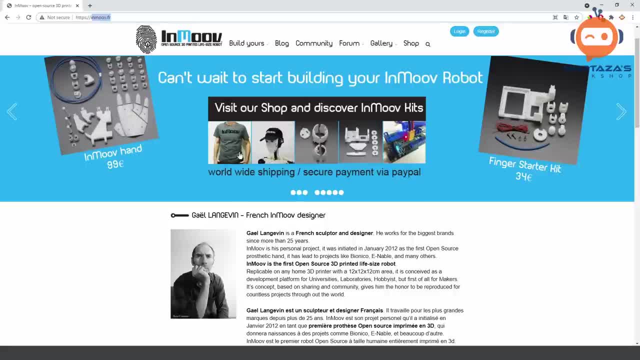 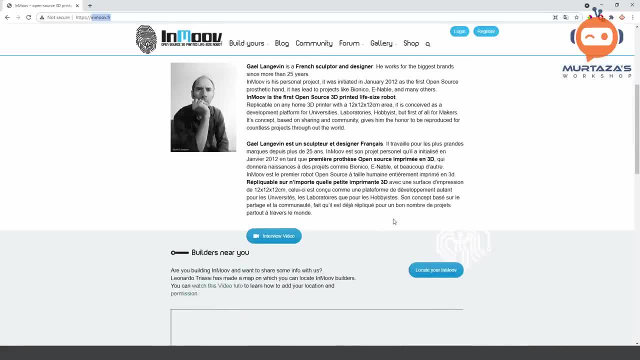 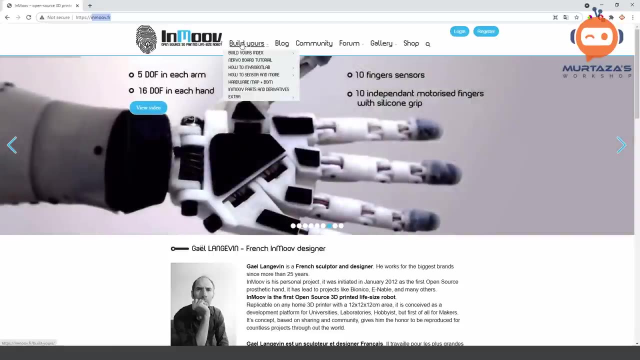 can see, this is the website in move dot fr and this is designed by a French designer by the name Gael Lagawin, So he designed this and he open sourced this for everyone to use. So thanks to him, And we can see that he has listed everything down. 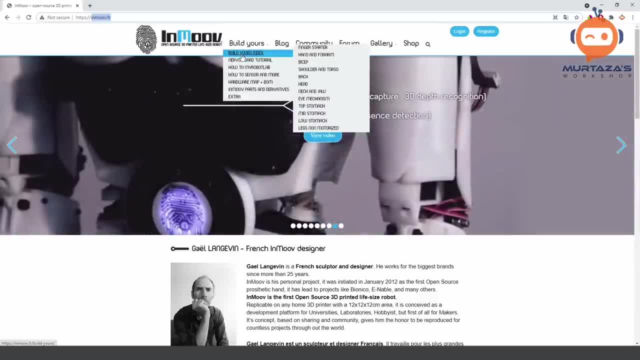 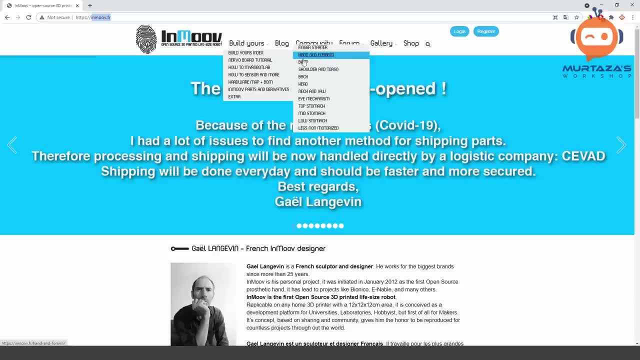 to make it easy for everyone to use. So here you can go to build yours, build your index, and here you can see finger, starter, hand, arm and forearm, bicep, shoulder and so on. So we will go to hand and forearm And here you are going to find all the steps to actually 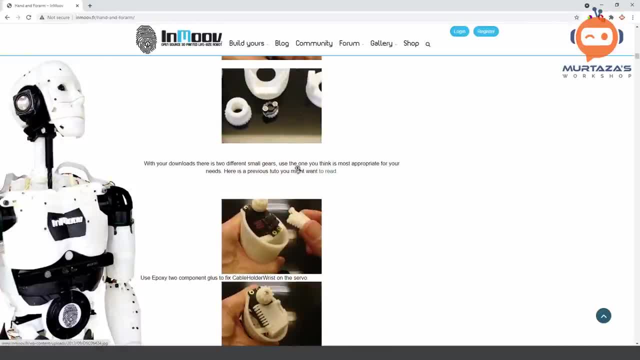 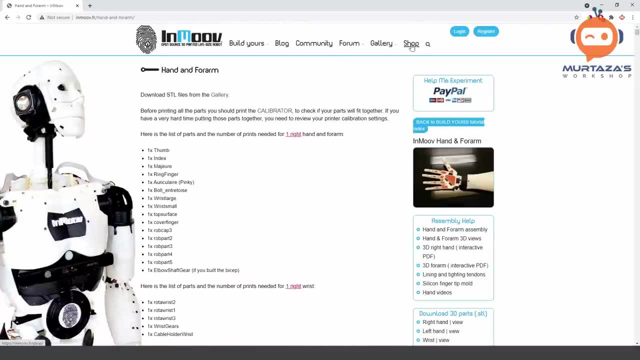 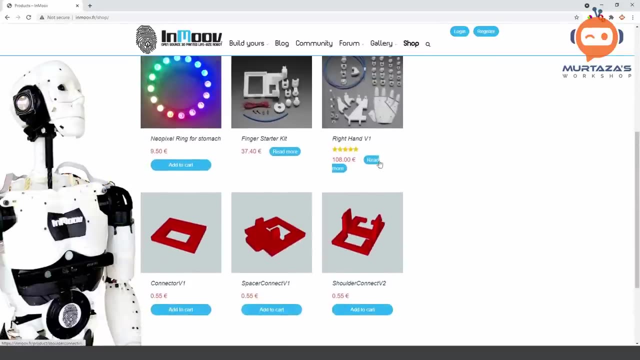 create this, And you can also find all the 3D printed files within this website as well. And if you don't want to go through all of this, do check out his shop as well, And there he's also selling this arm if you want to purchase that. So at least he's selling the hand rather. 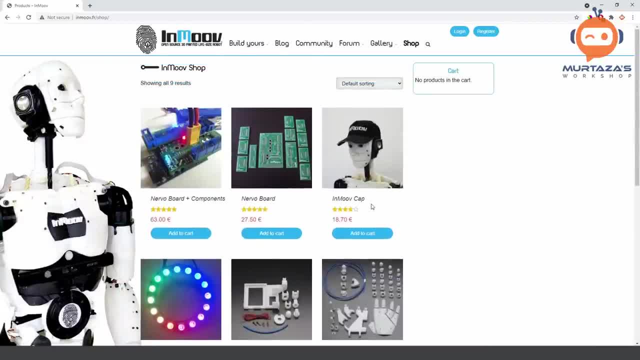 than the arm. I believe there was arm at some point as well, I'm not sure. Anyways, you can get a cheap printer and you can print it yourself, And nowadays printers are very, very cheap and you can easily use them right out of the box. So we are going to build this. 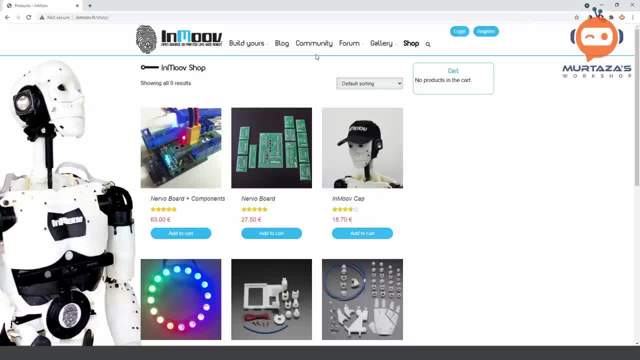 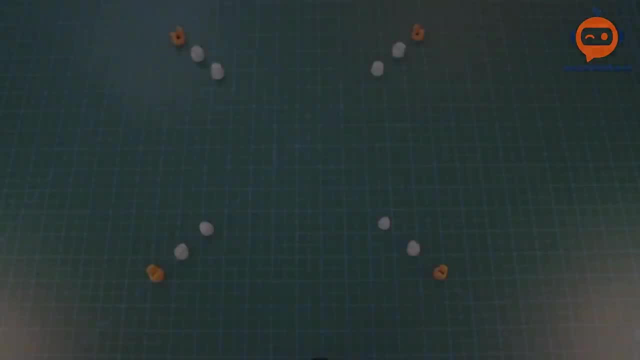 Now I printed this almost one year back, So I will show you all the process of how I did this, And then later on we are going to look at the electronics and then we will go on to the coding part. Here we go. 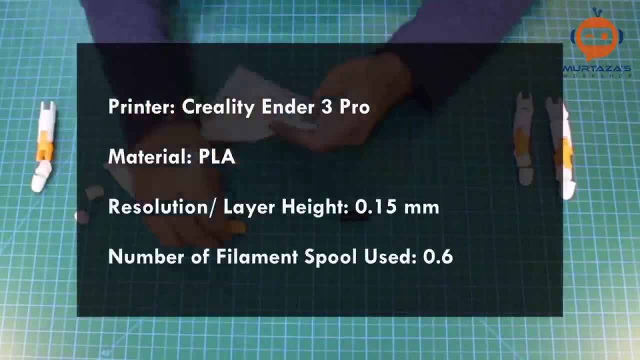 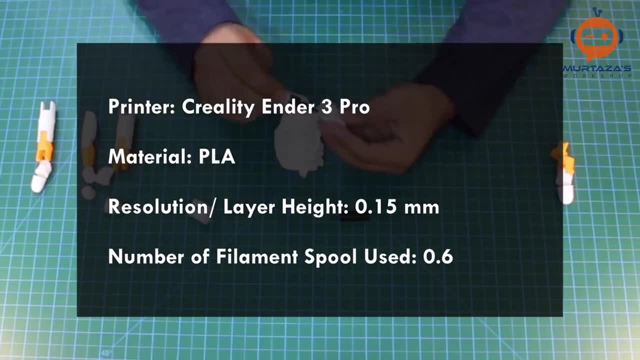 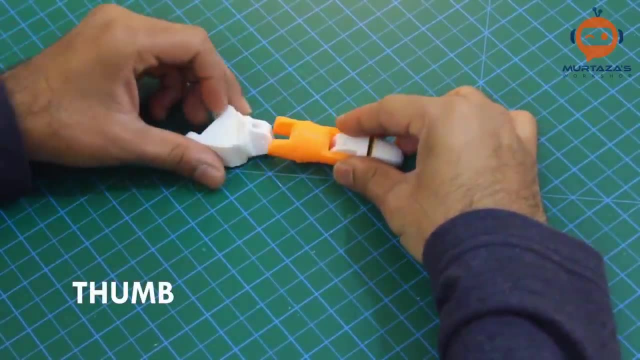 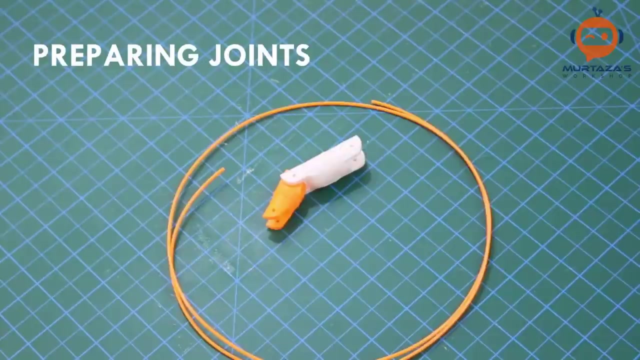 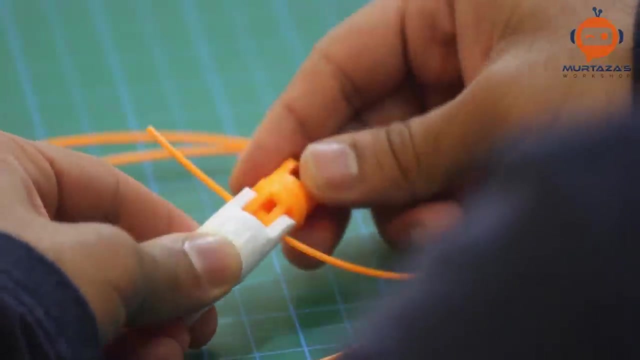 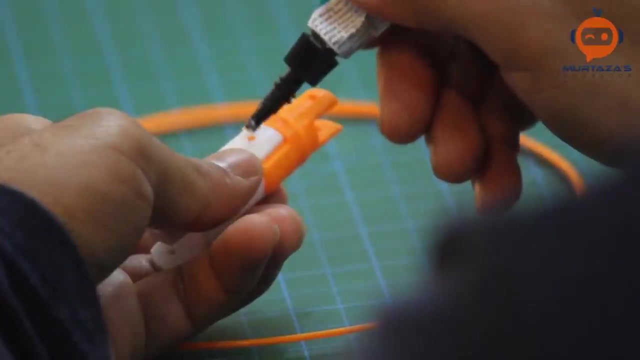 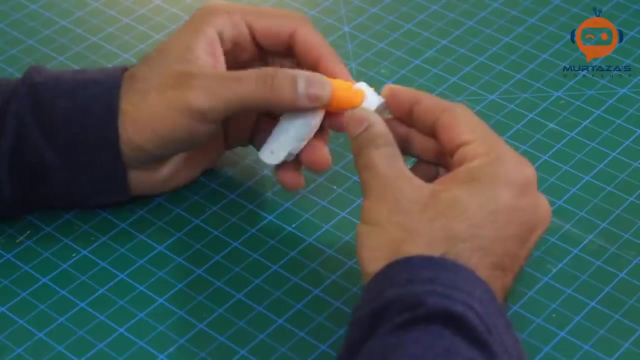 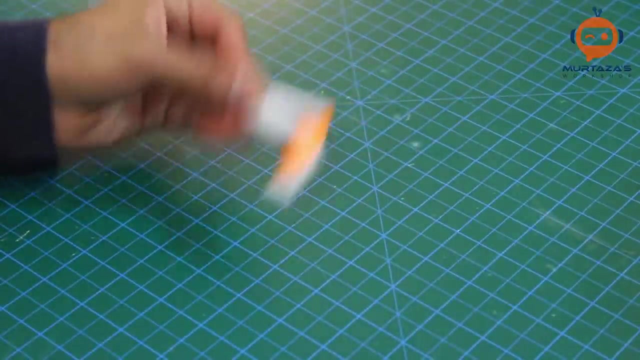 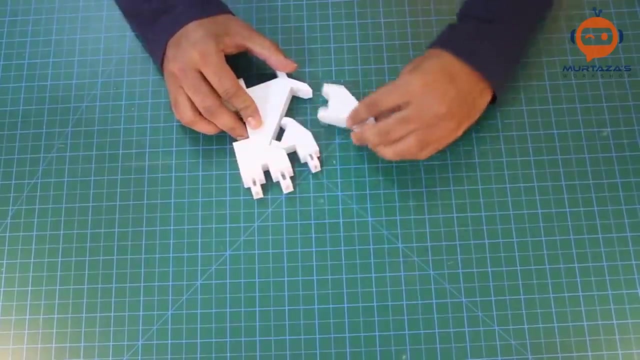 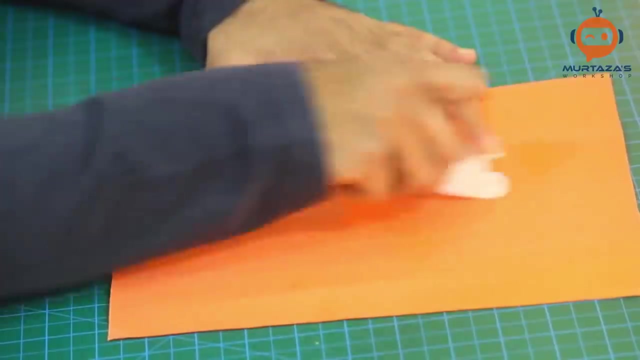 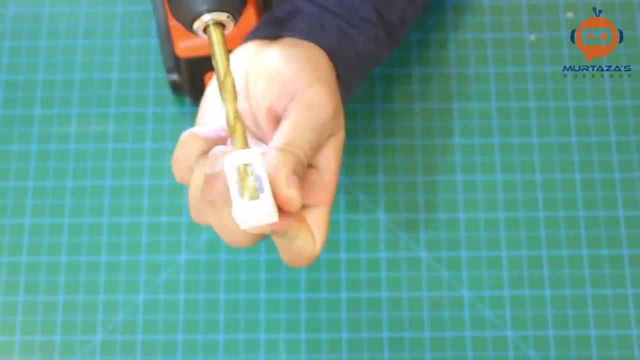 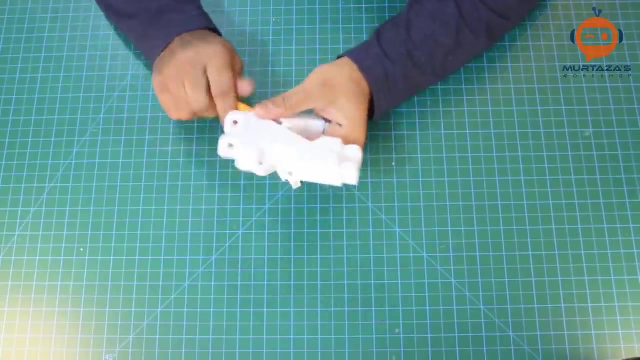 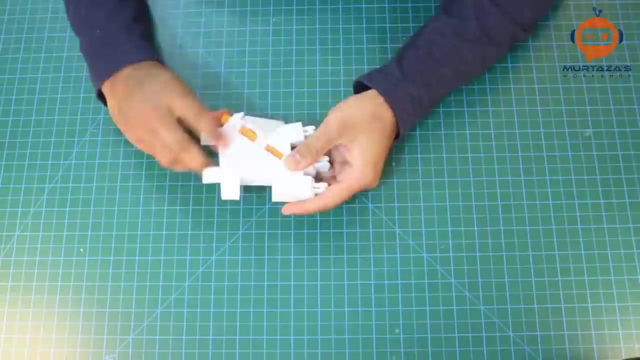 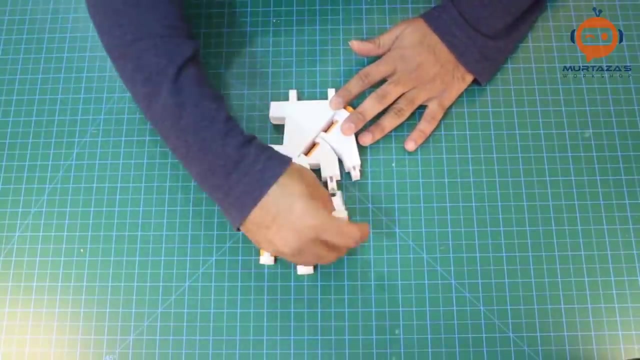 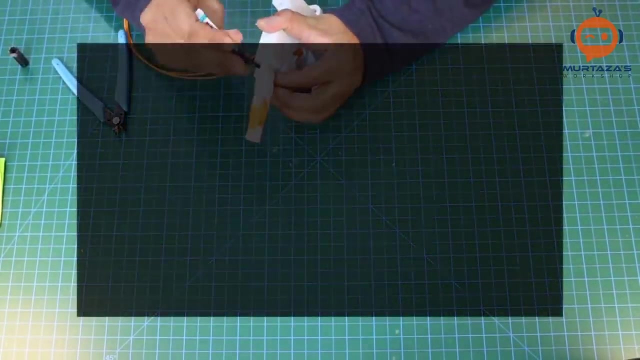 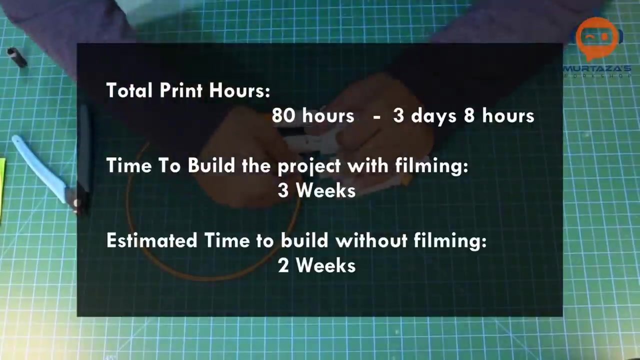 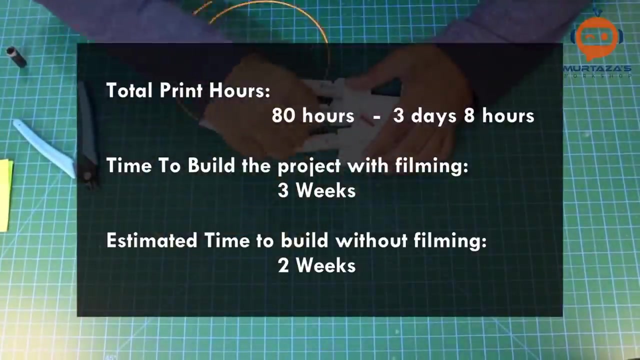 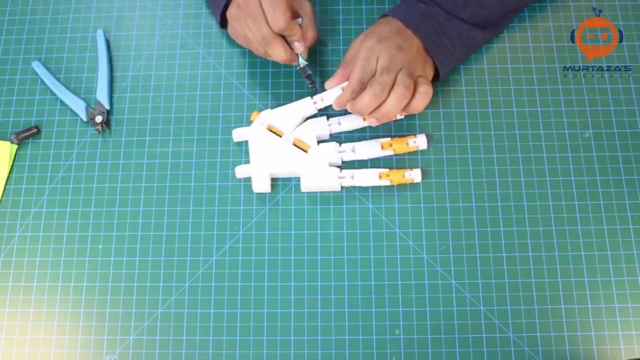 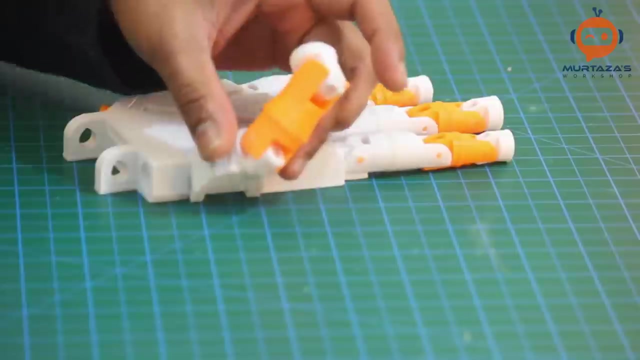 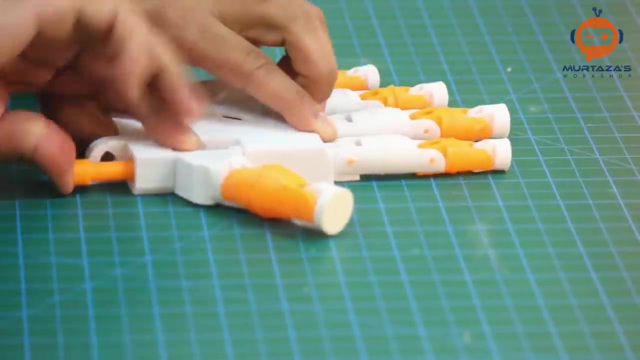 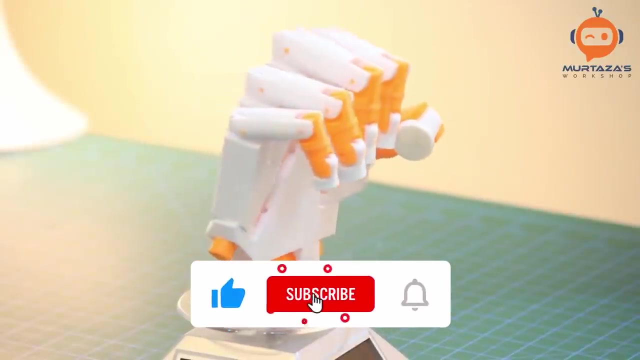 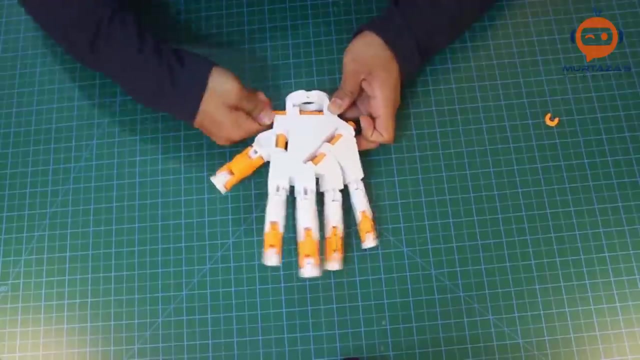 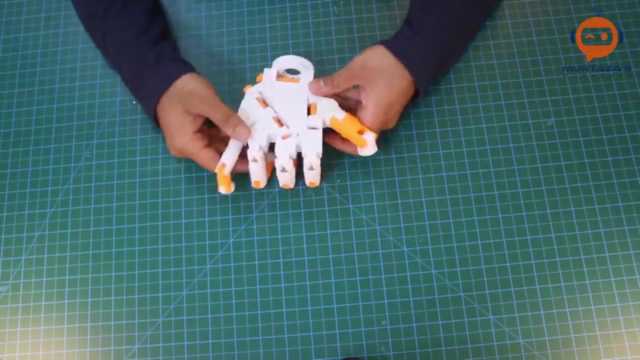 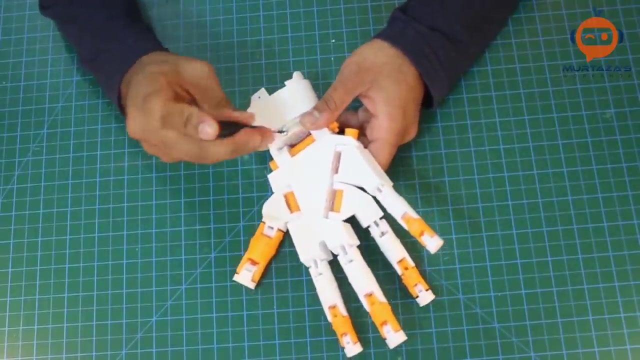 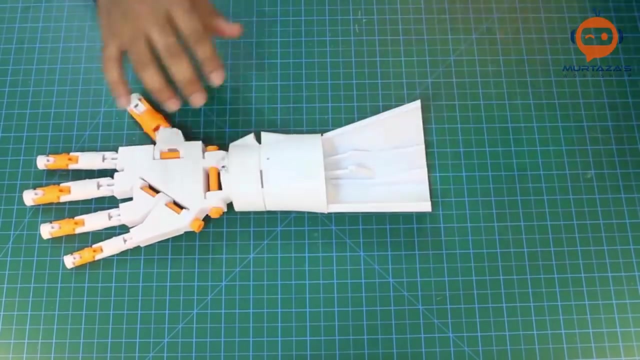 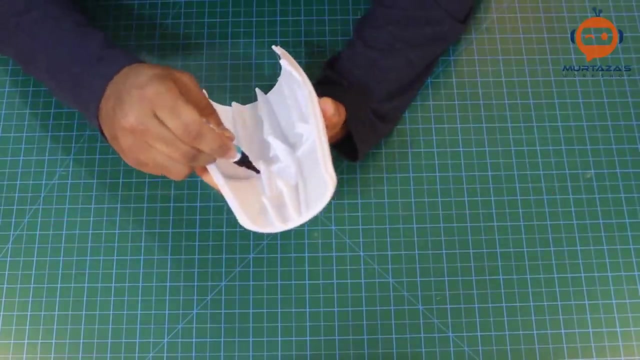 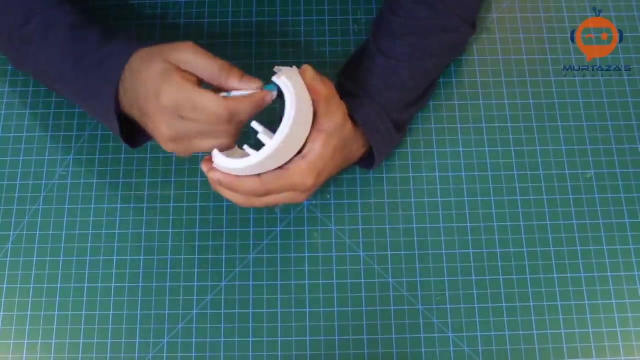 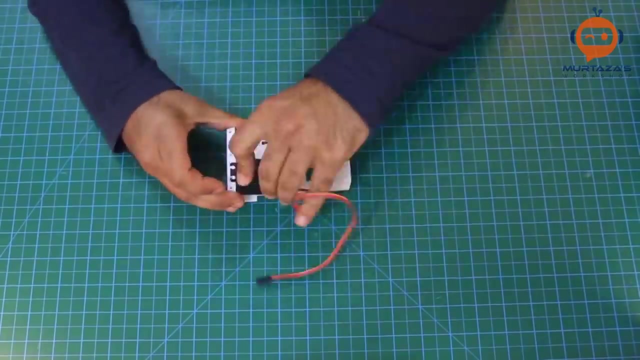 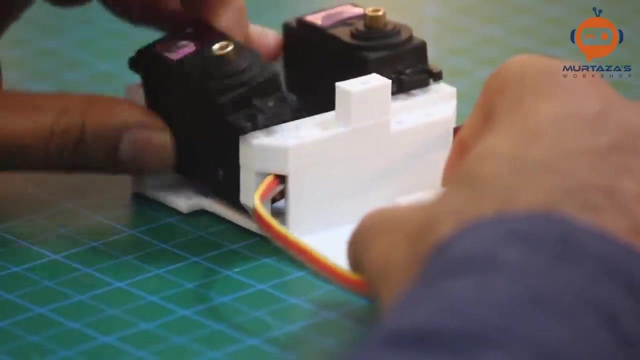 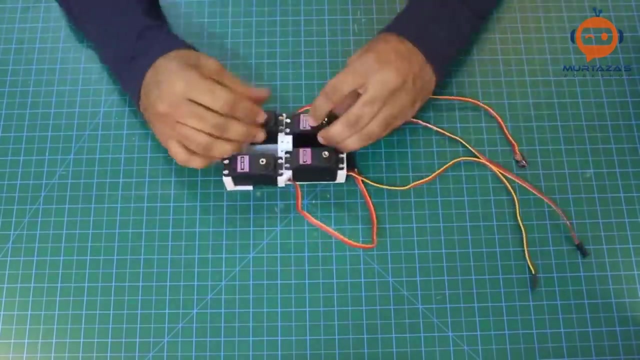 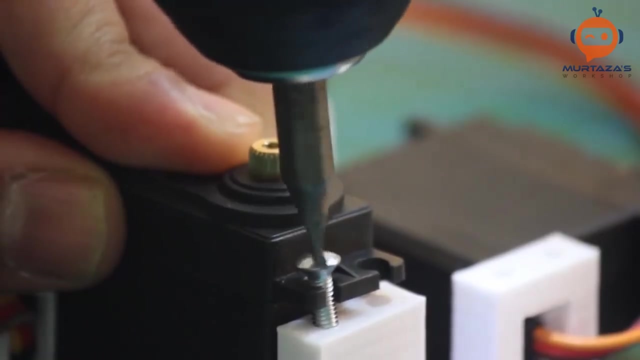 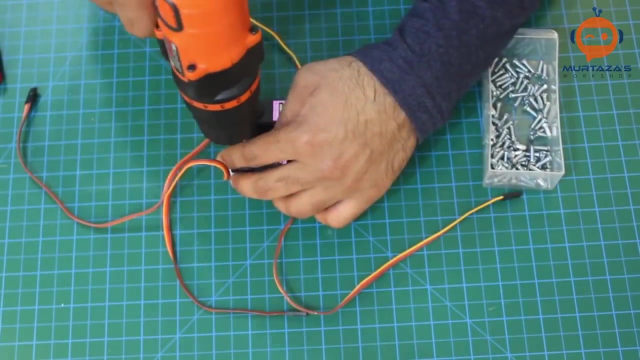 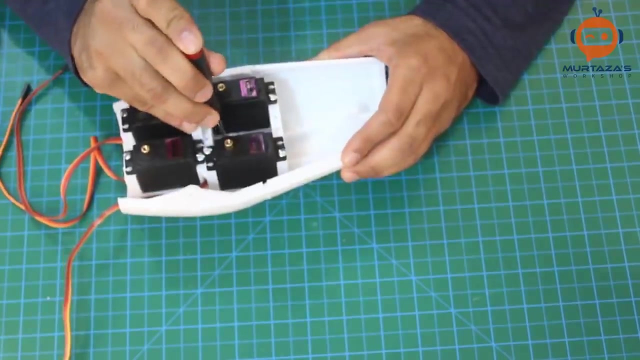 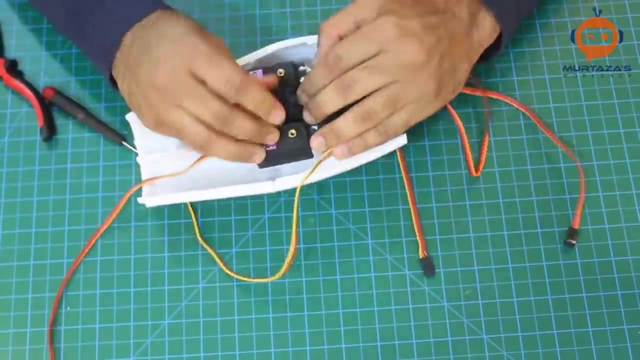 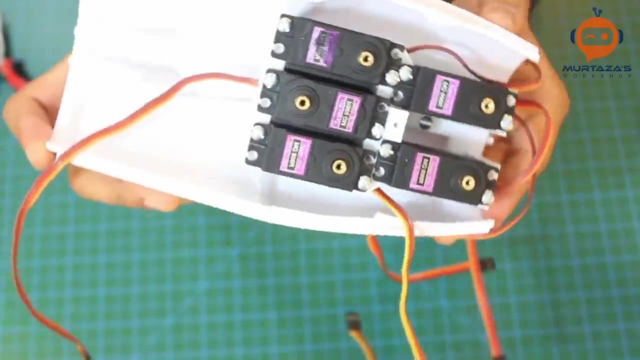 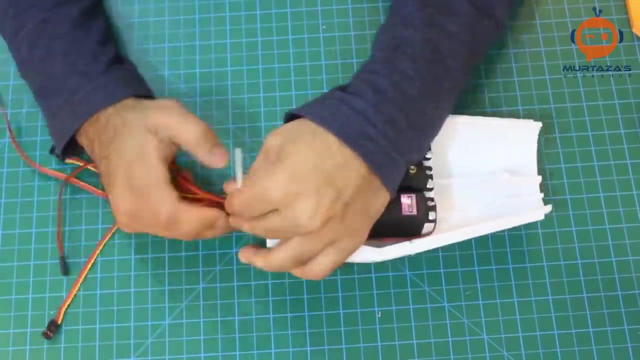 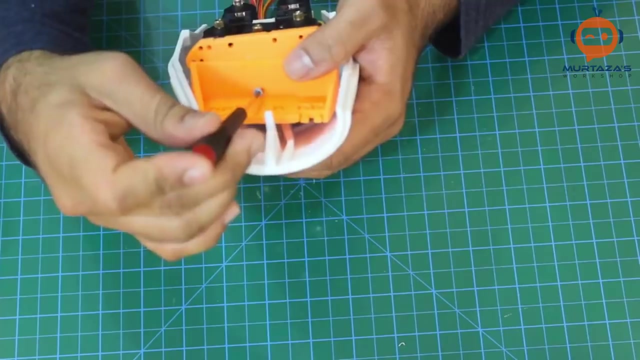 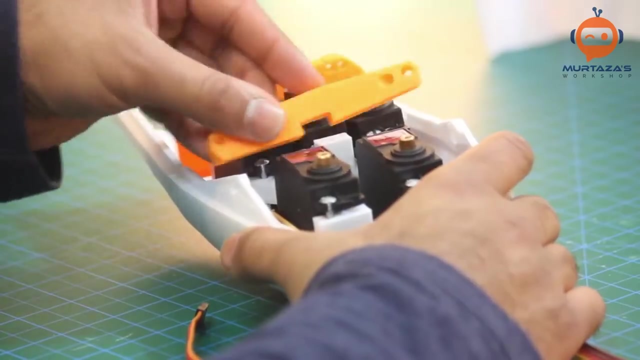 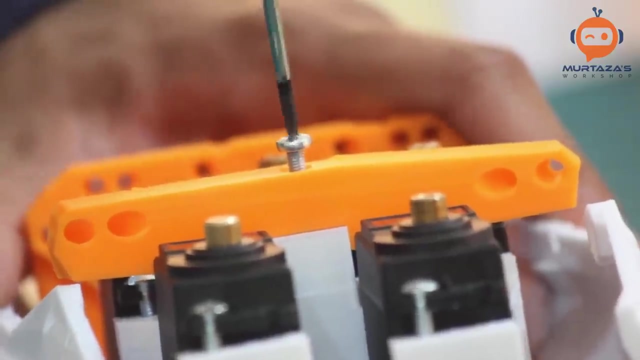 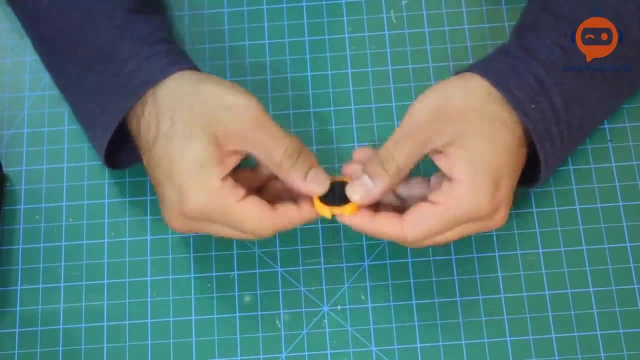 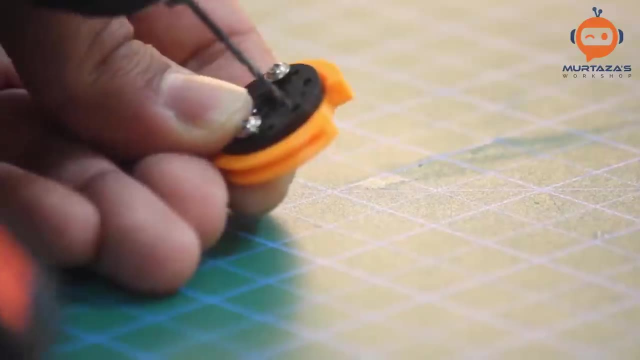 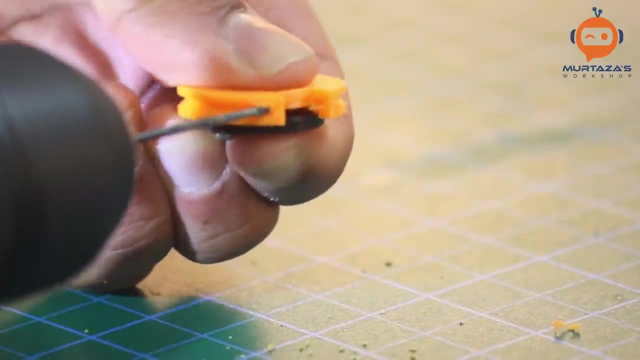 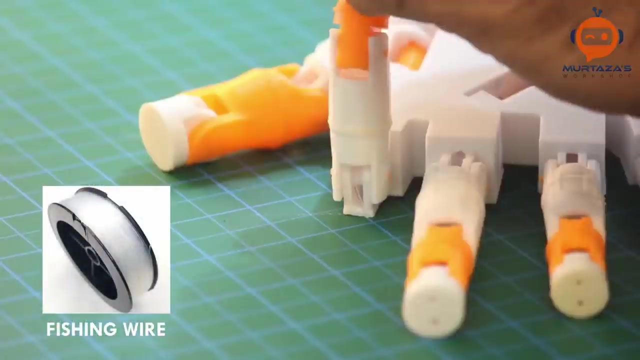 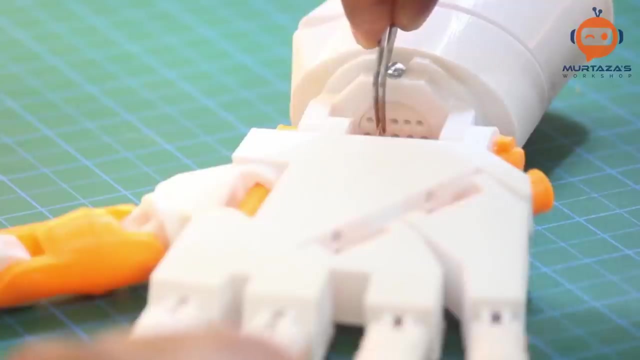 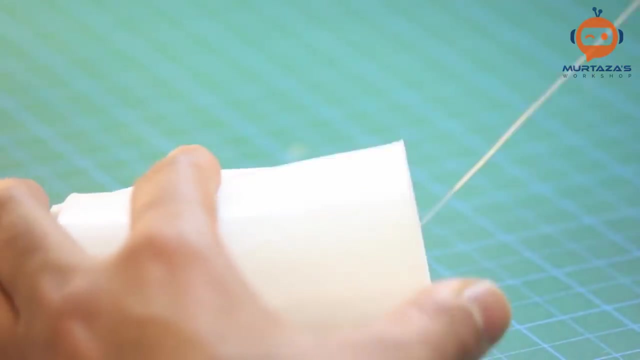 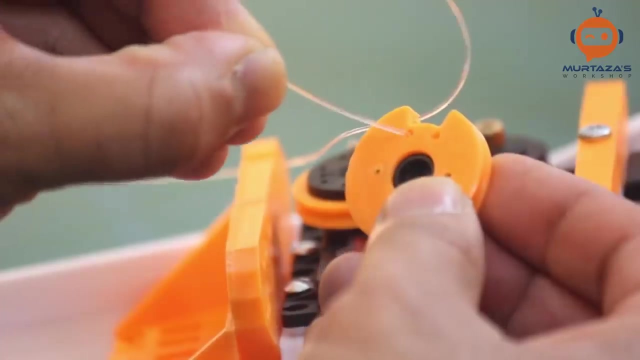 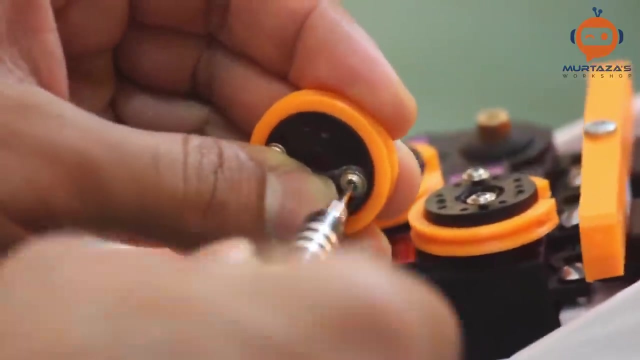 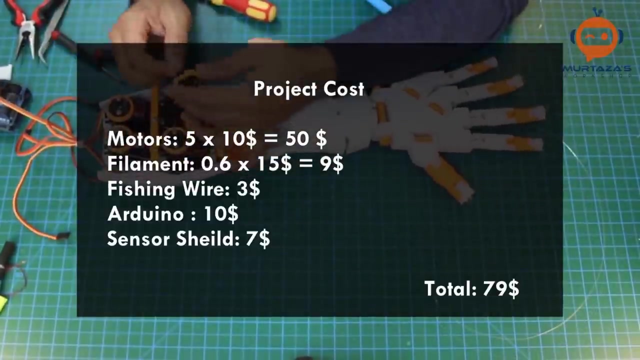 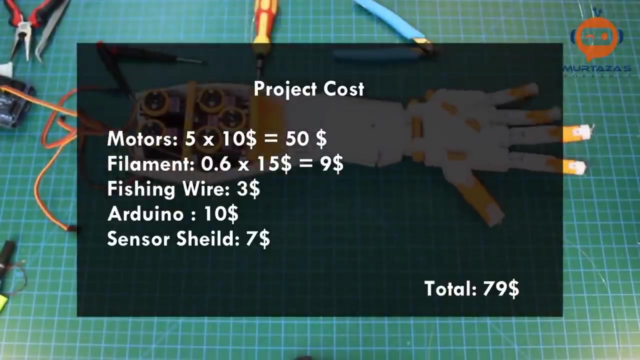 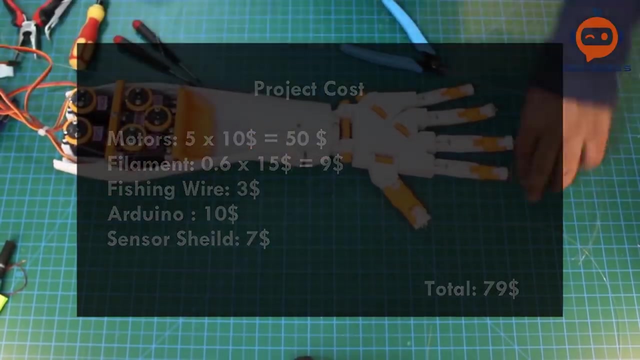 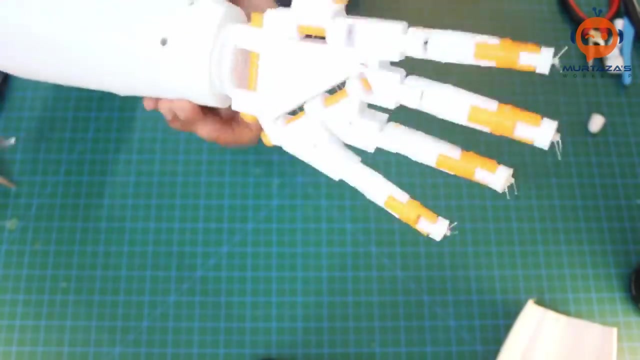 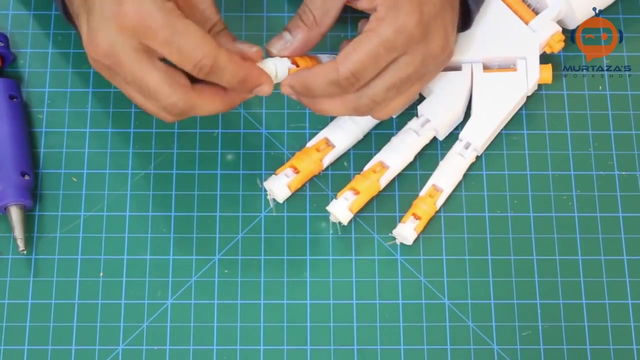 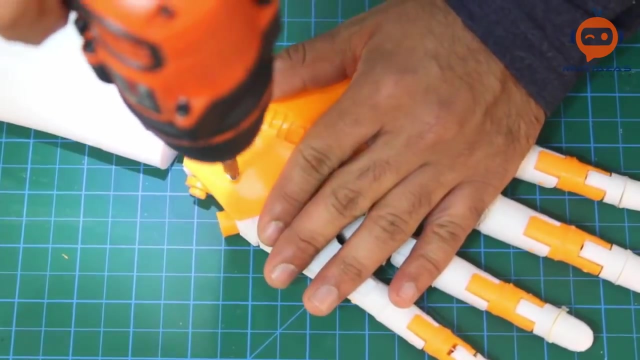 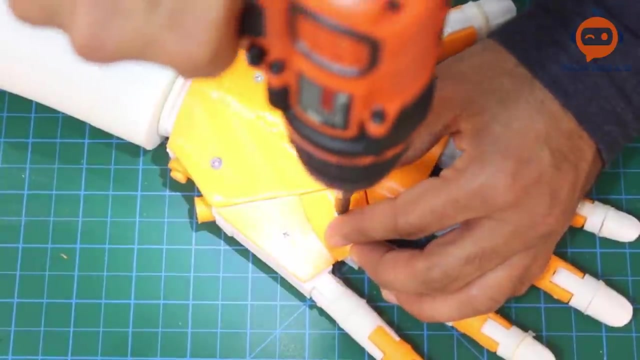 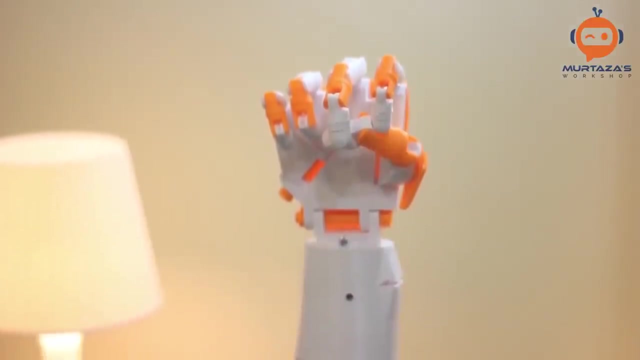 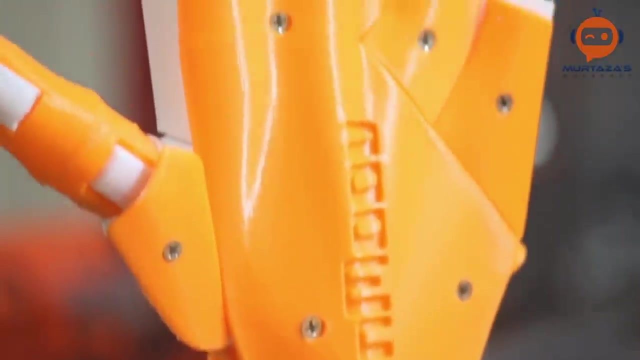 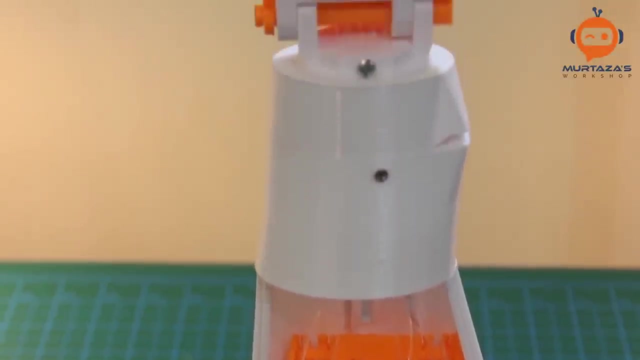 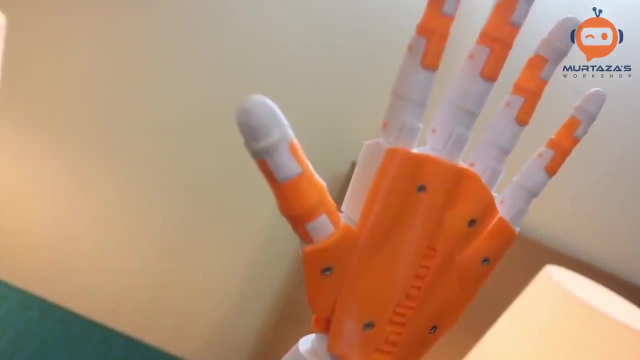 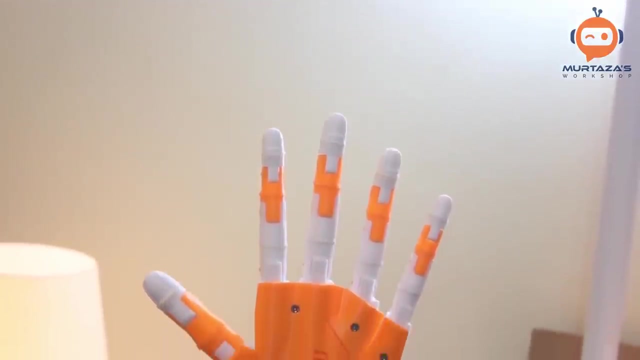 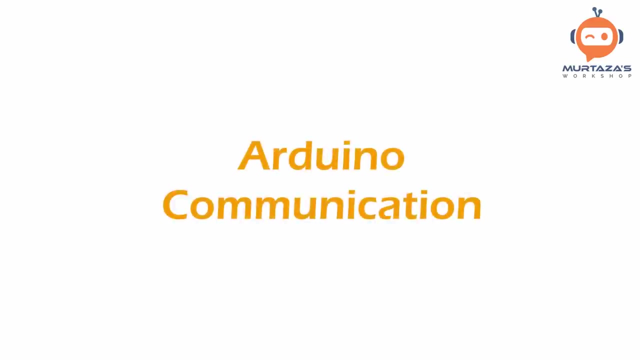 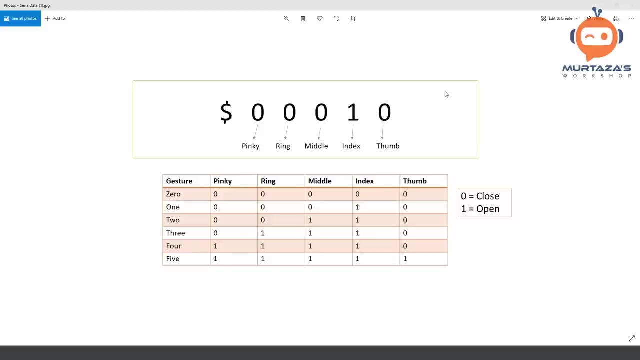 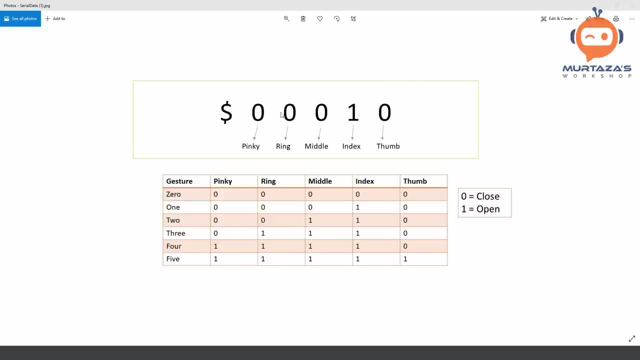 So the idea is fairly simple. We are simply going to send zeros and ones based on which finger is open and which finger is closed. So whenever a finger is open, we are going to send one. So, as you can see here, and whenever it is closed, we are going to send zero. 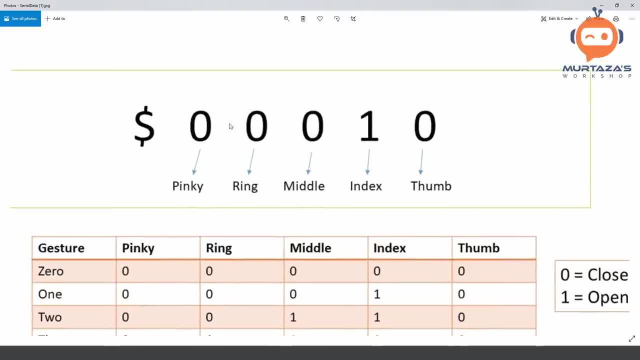 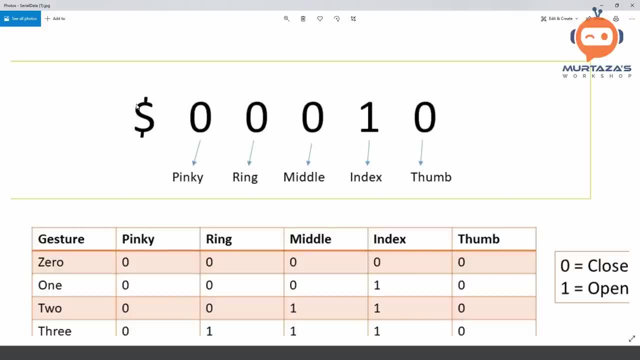 So the string that we will send from our Python code will be 0, 0, 0, 0, 0, and then it will have a dollar sign in front of it. so at the starting it will be a dollar sign, and then you have these five digits corresponding to whether each finger is open or 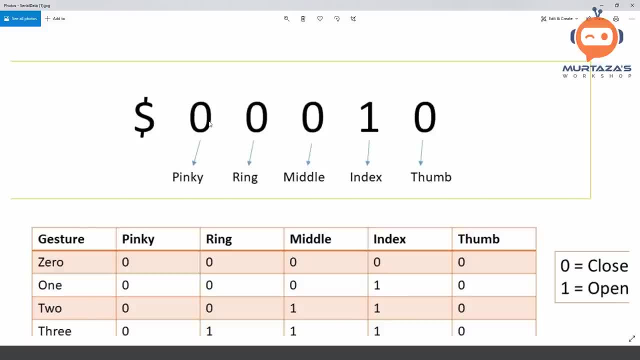 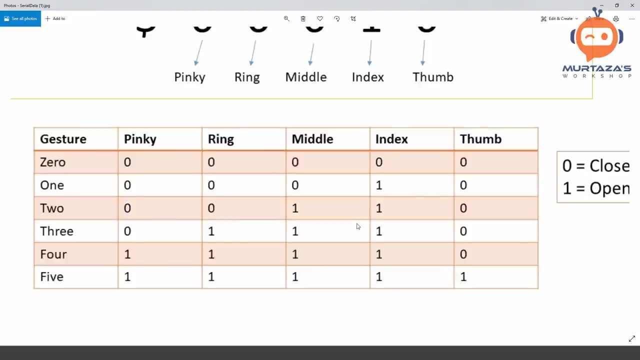 closed. so if, for example, pinky is closed, it will be zero, if it's open, it will be one. now, in our previous project, the last time we did this, so earlier, we had the issue that if we open any finger, we cannot tell which finger is open. we just open one finger, the index finger, and that's. 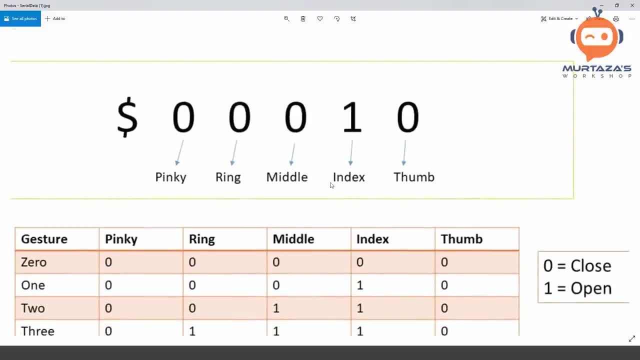 it. so in this, in this scenario, we are not going to do that for each individual case. we are going to open and close, so you can literally make any sign or anything with your hand and it will represent that exact same gesture with the, with the robot arm. so this is a kind of an upgrade, and 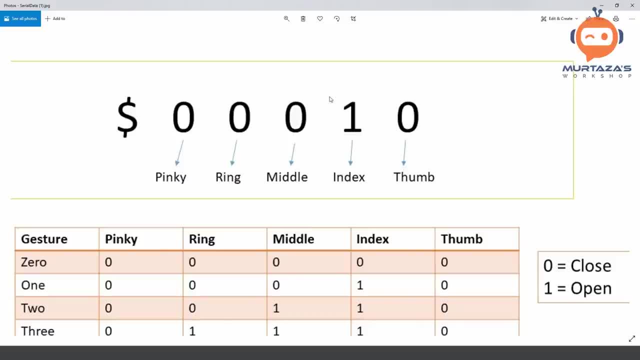 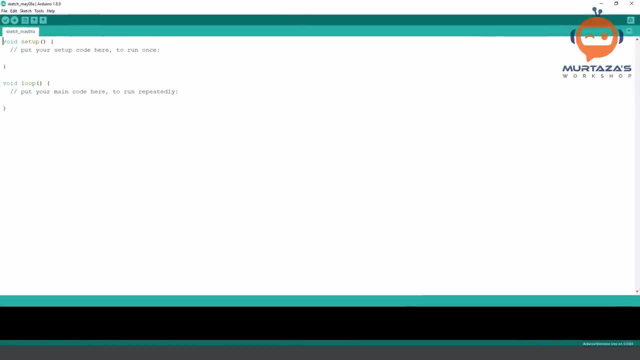 it is much faster than what we did before. so this is basically the serial communication idea. so what we will do is we will open up our Arduino, and here let me make it a little bit bigger so you can see better. so here we are going to first of all save this, so we will write here. robot arm finger counter gesture. 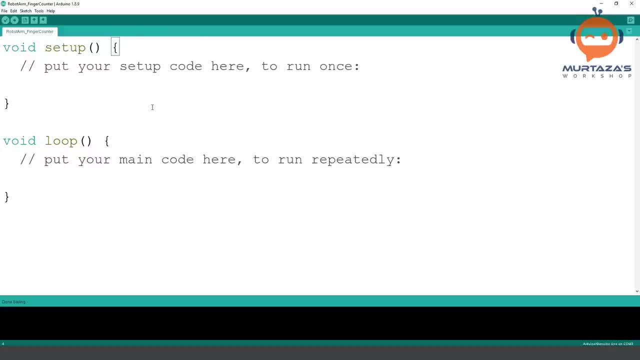 whatever you want to write, you can write here and we will save it now. first of all, we are going to include, uh, or let's do the serial part first, then we can go on to the servo part. so first of all, we are going to write here: integer values. 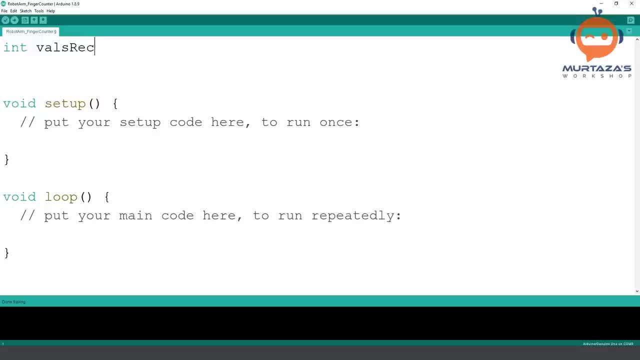 receive. so whatever values we receive, we are going to put them in an array, and this array will be the number of values received. so we are making it a variable so that if you wanted to use it in other projects, you can do that too. now, in order to use a variable like this within an array, in the definition we will have to 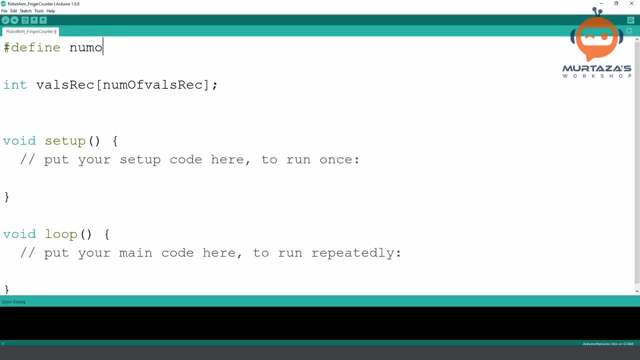 define here. define number of valves receive. why is this v small? we are using camel casing, so we will use it like that. okay, so this is the number of values received. so we are going to define here. this is the idea, so then we can put the value here that, for example, in this case we are receiving. 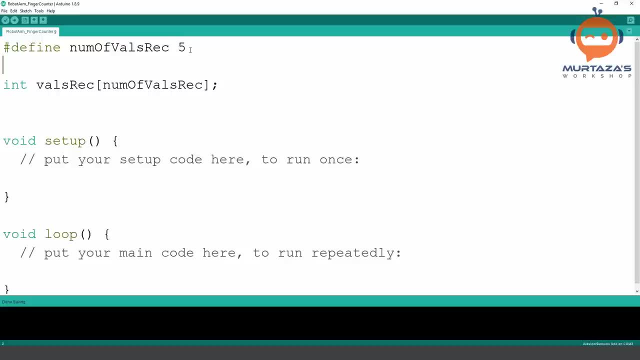 five values, okay, and then we also need to define one more thing, which is the digits per value received. now, the good thing about this code is that you can use it later on as well for other projects. so, for example, if you are receiving, uh, let's say, a value from the analog sensor, 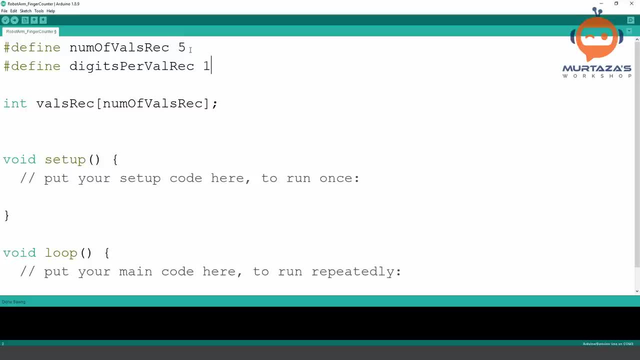 which has a range from 0 to 1000, then you can have four digits. so here instead of one, you can just write four. and let's say you have three sensors connected. you can write: here: we are receiving three values from three different sensors. so it makes it very easy to work with different projects. 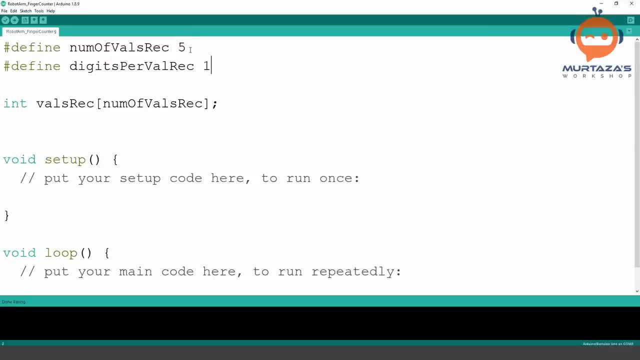 that's why we are writing it like this, but here for now, we are going to use five and one. okay, so once that is done, we are going to define our string length. so our string length will basically what we are referring to is that dollar. then we have zero, zero, zero, zero zero. so this is our string. 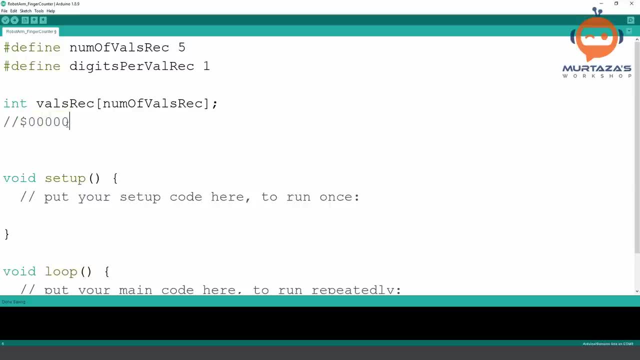 length, which is zero, one, two, three, four, five. so how can we do that? we can simply calculate it, because we have the number of values receiving and we have the digits per value. so we can simply calculate it. so we can write here: integer string length is equals to number of values received multiplied by digits per val value, or val received plus one. 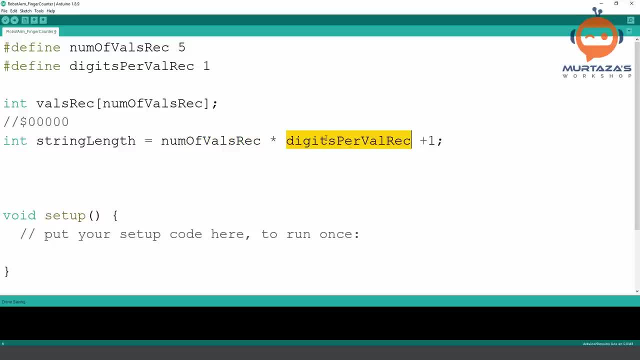 so here, basically, we are saying we multiply this with this, and that will give us all these, which will be five, but then we also have a dollar sign, so we will add plus one. so this is what we are doing so far. so very simple, very easy. let's put it here. there you go. then we are going to initialize. 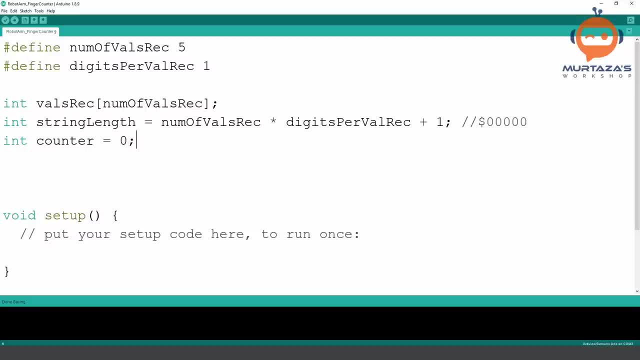 a counter. this counter will be used to actually see or iterate through all these different characters. so we will be using that later on and then we will also initialize a flag which will be counter starts, and we will keep it as false. so whenever we receive the dollar sign, this dollar sign. 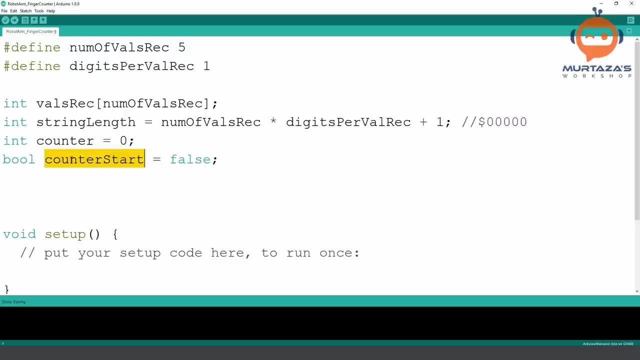 we will start our counter. so that's the idea. and once we start the counter, we are going to keep adding to our counter. we will do plus, plus and that will keep adding to our counter and we will know: uh, we have to go till this string length. that's why we are using the string length as well. 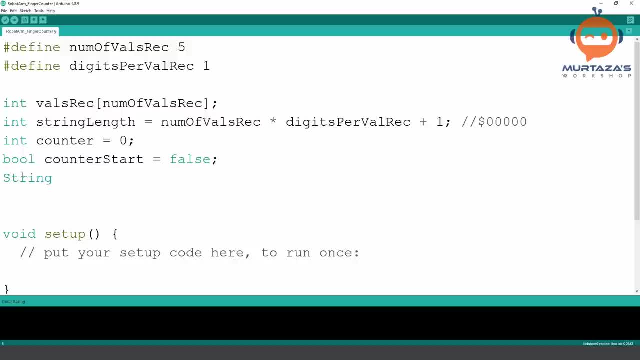 okay, then we will add a string. this string will be received string. so when we receive the string, basically what we are doing is we are collecting it all together and then we will break it down into substrings, and these substrings we are going to store in our value received. so it might be a little bit confusing at this point, but don't. 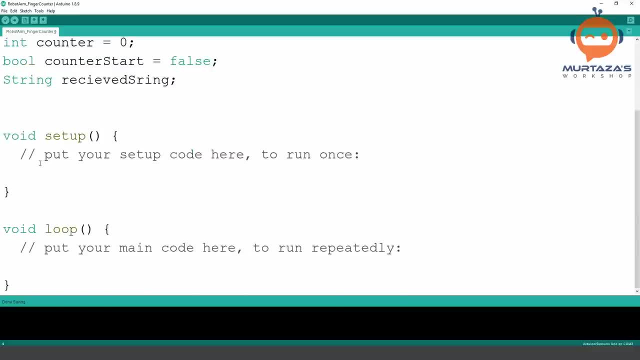 worry, when we go ahead, i will explain everything. step okay, then in the void setup, do we need to initialize anything for the serial? yes, we need to write serialbegin, serialbegin, and we have to write the bot rates 9600. and then what else? then for now we don't need to do anything else here and then we can skip the loop for now. later on we can. 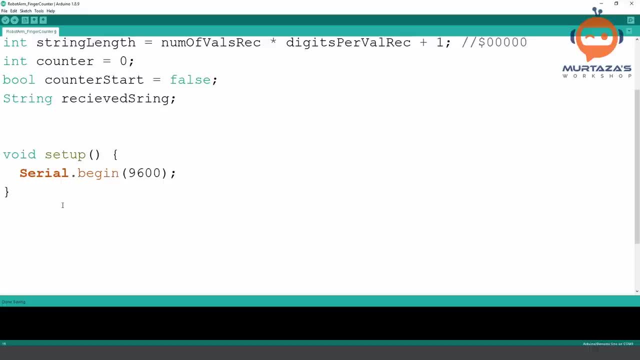 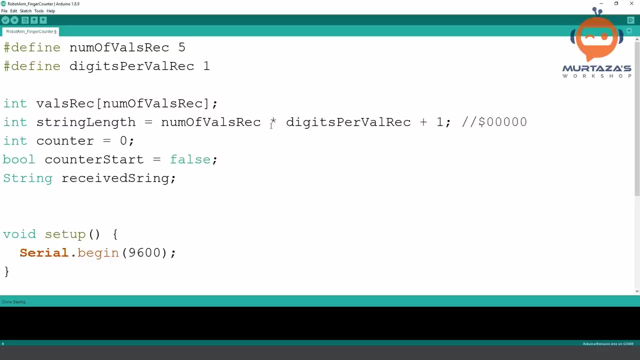 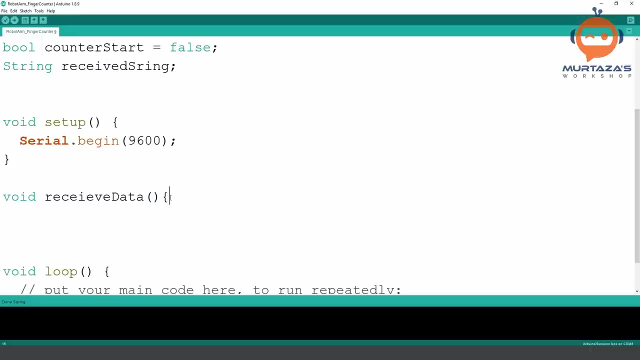 use it. here we are going to create a new function. we do not, uh, intend to output anything or return anything, so we will write void. we will write here: receive data- uh, i believe i wrote the spelling here wrong. receive this ring, okay. did i write anything else wrong? um, not so far, hopefully, okay. so then we will. 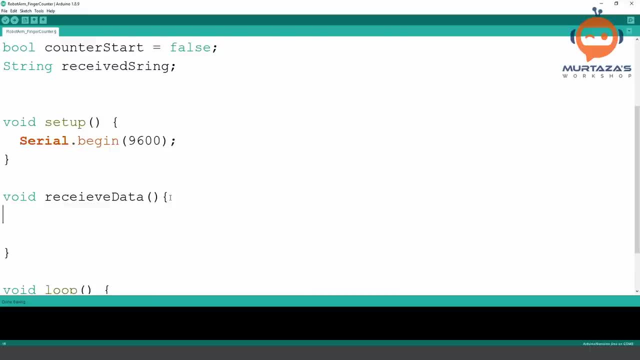 add our brackets to start and end, and then we are going to write while while serialavailable available, then we are going to go ahead. okay, so we will write pretty much everything here inside this, okay, so what is the next step? step? the next step is to read the character, so the the data that is coming. 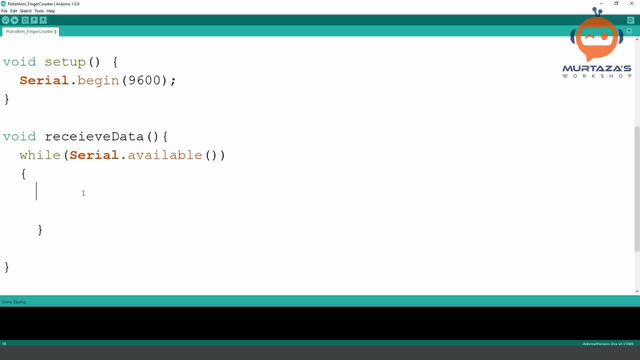 from the Python script is not actually as a complete string. it will come a character by character. so we need to read each character. so we will write here: character C is equals to serial dot read and we are going to read this character. then we need to check if our character is dollar. so this is the 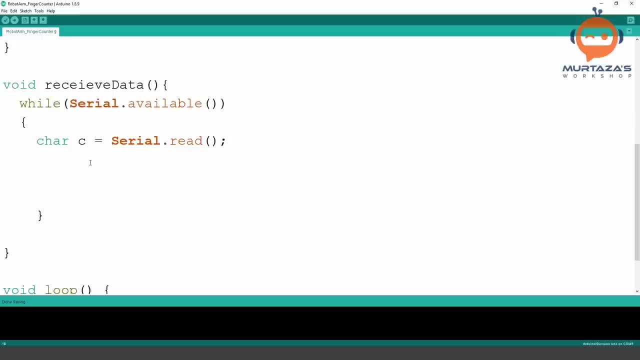 character we are looking for. so we need to check here that if the character is equals to dollars, then we are going to say counter: did I put a bracket? because we have a lot of brackets, it can get confusing very easily. so here we will write: counter starts is equals to true. so now this counter will start and 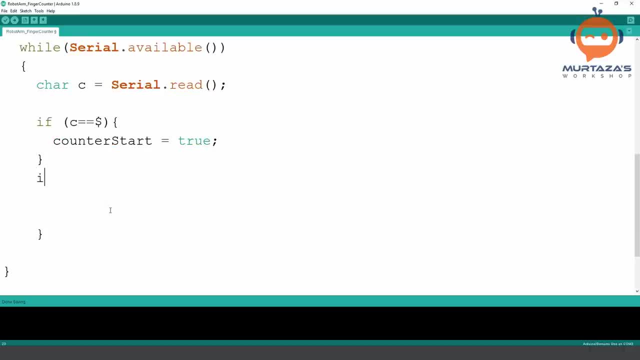 then we need to check if counter starts, this basically means is equals to true. we don't need to write that. if we just leave it like that, it means the same thing, and then then we are going to check if we have reached our string length. so we will write here if 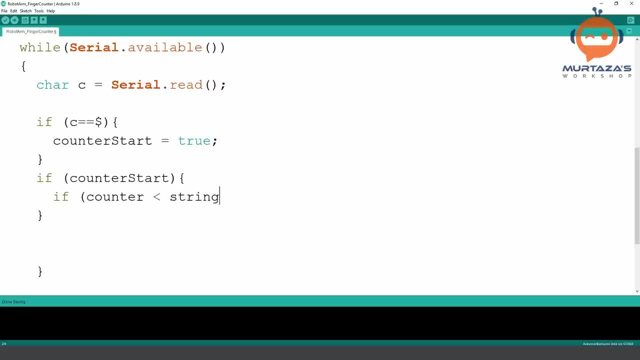 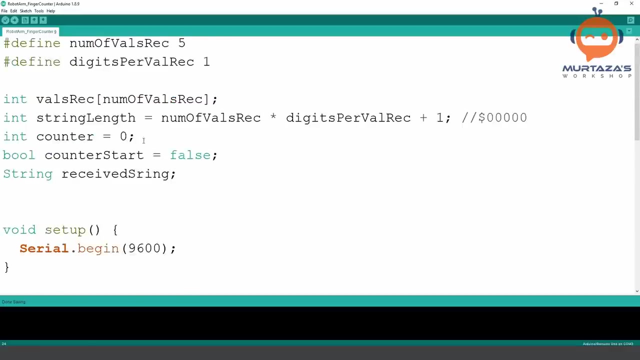 is less than our string length, then we are going to count. right, so we will do the count plus, plus and all of that. actually, let's put them together. we can format that later, okay? so basically what we are saying is: as long as we have not reached till the end, keep counting one by one, and each time we are going to get. 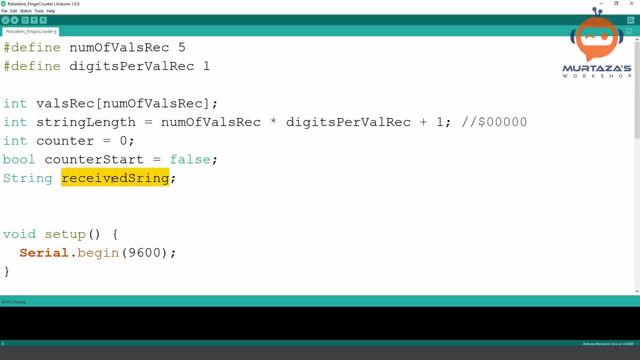 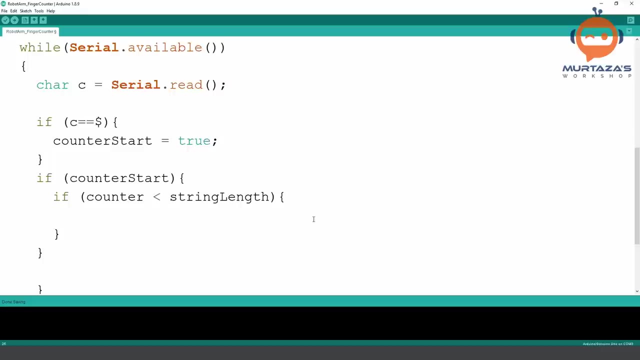 this string and we will add it to this string. sorry this character. we will add to this string. okay, the spelling here is wrong: s-t-r-i-n-g. okay, so what we will do is we will write here that our received string, our received string, is equals to. 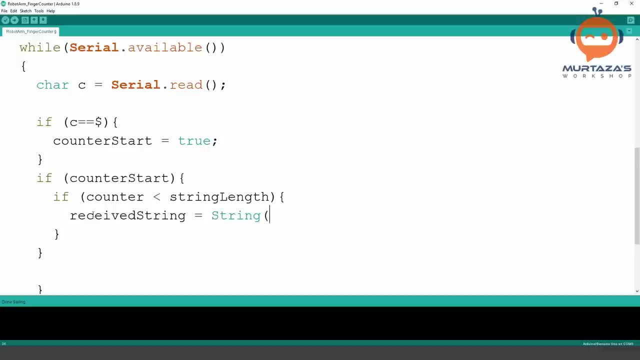 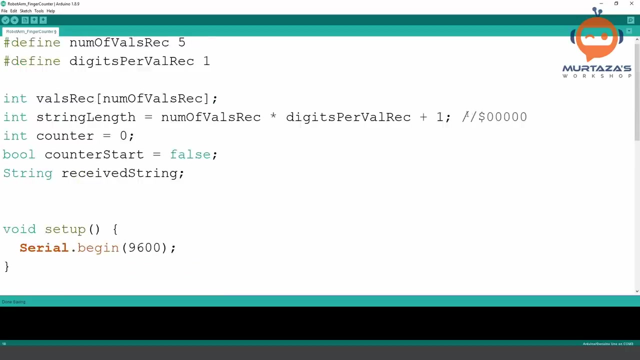 string, received string plus C. so what does that mean? that means that whatever our received string was earlier, so earlier it is nothing, so it is empty. so we will add our string to it, our character to it that we received just now. so it could be dollar sign, it could be the zero or one, whatever it is, we will add to it. and 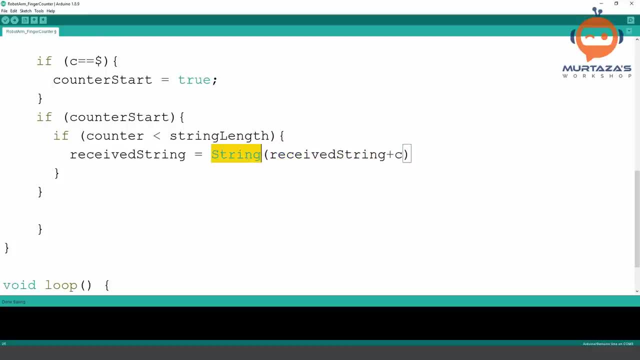 then to make sure it is string, we will write here string, so that is the main idea. and then we need to add to our counter. so we will say counter plus, plus, so this will add to the counter and it will keep iterating. so this is as long as this statement is not reached, so then we can write here: 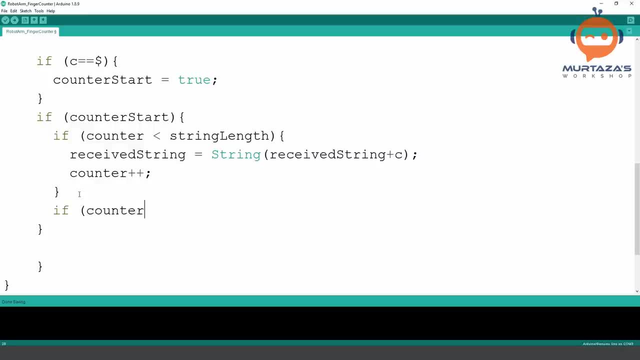 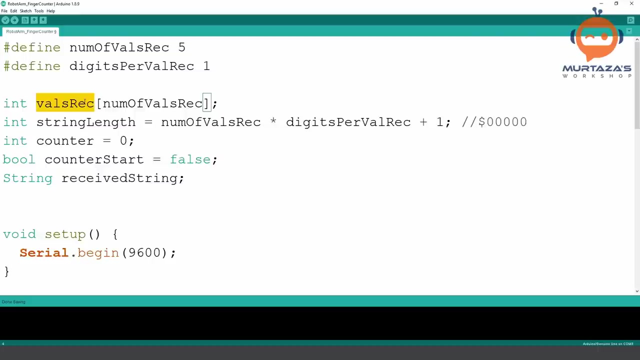 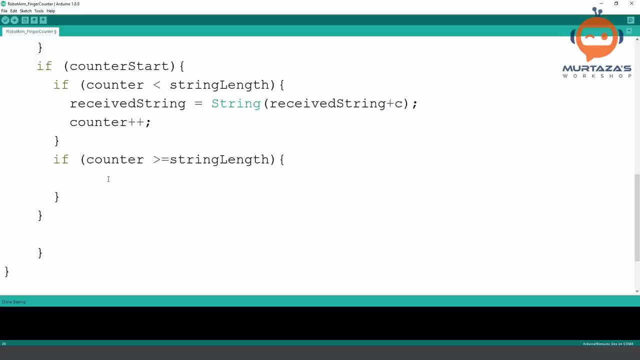 that if our counter is greater than or equal to string length, an Array, Then we are going to actually store our values in where is it? in the values received. so this, we will store it in this array. so here we are going to write. so how do we actually put it in this array? let me explain. we can write here: 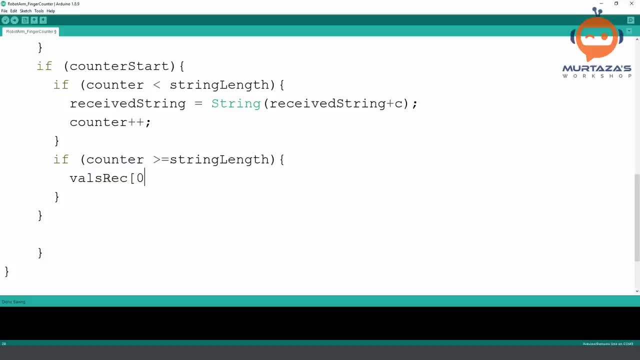 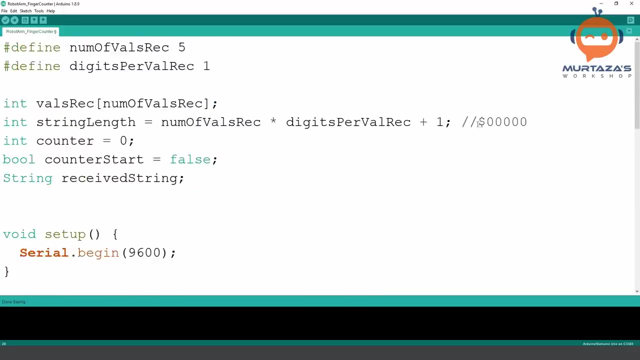 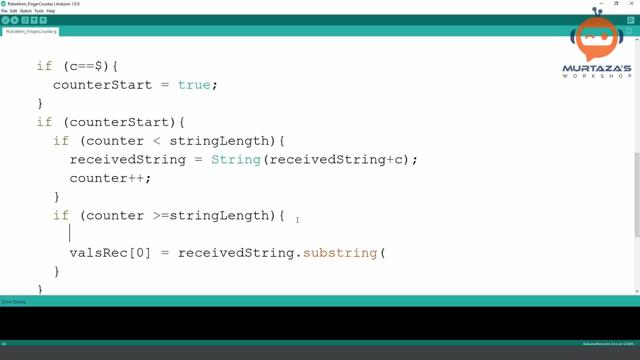 values received, let's say at zero, is equals to, to our received string. received string dot, substring, so we can write substring and then this is basically a function, or you can say, a method that we can use to actually split our string. so right now, at this point, our received string is basically this and what we need to do. 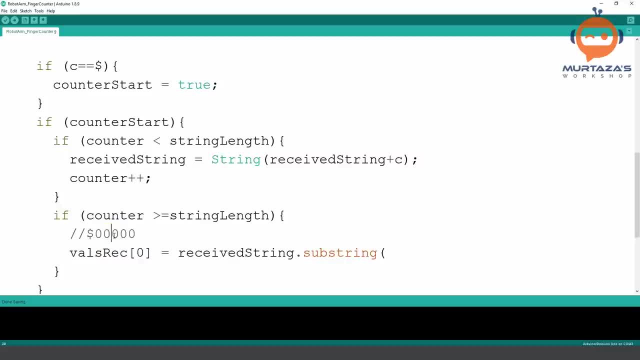 is we need to go ahead and split it one by one, like this: so we will give it some values. so we are going to say that, for example, start from zero and go till one. so we can say it like this. and then what we will do is, because these are numbers, we can put dots to int because later on, 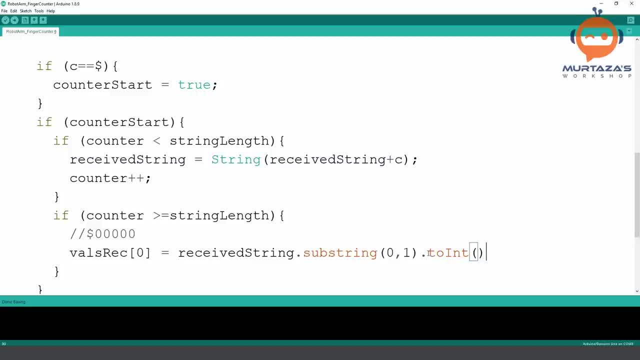 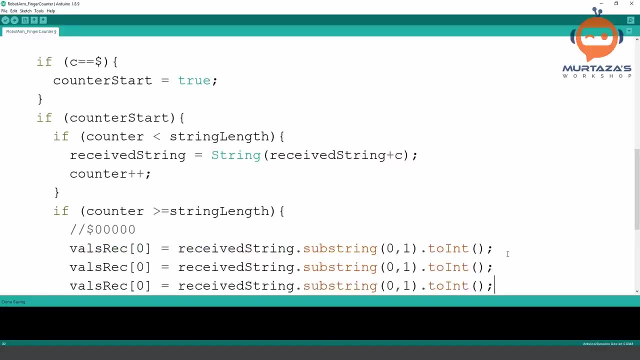 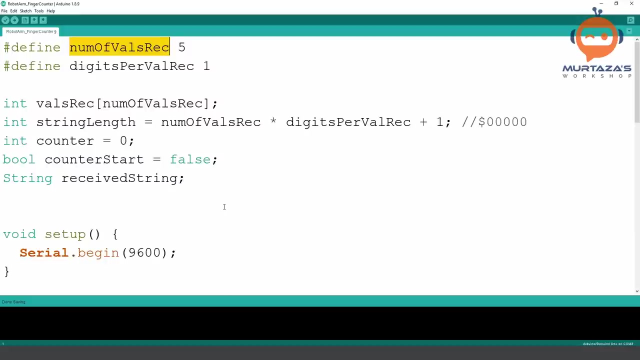 we are going to use these values to send command to the servo, so we need it in integer rather than string, so we can write it like this. but the problem here is that i will have to copy this and i will have to paste it five times because we have five values that we want to receive right, so i will have to 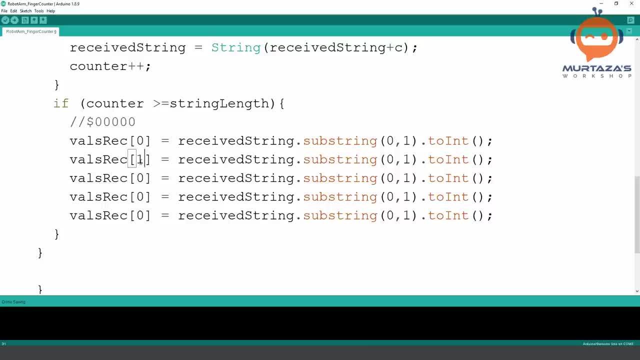 paste this five times and then i will just change this value to one, two and so on, and i will change these numbers to one and two and so on. but there are two problems here. one is that let's say i have more than five values then once. then i will put more, that is, 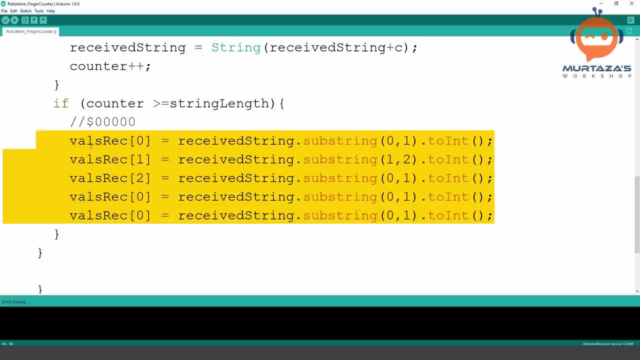 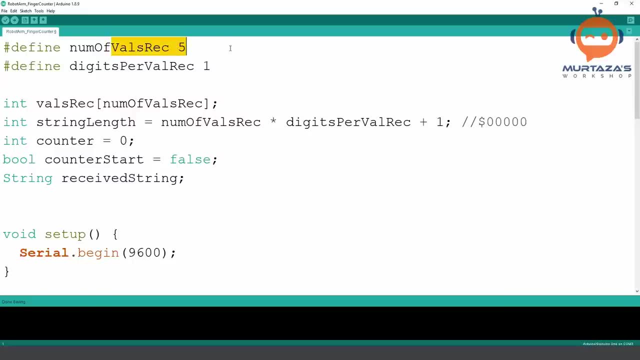 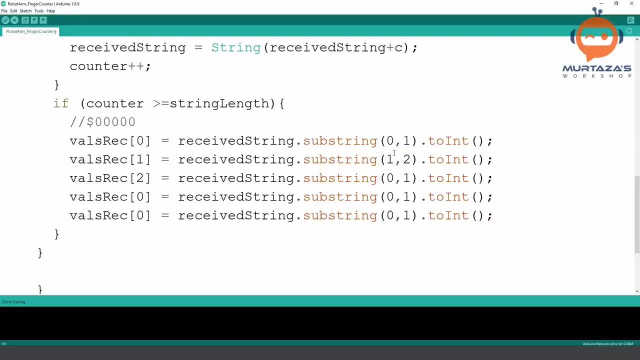 not a good way to do this. that is kind of hard coding. so what we can do is we can use a for loop, so the for loop will loop as many times as we have the values, and the second thing is we need to update these values. so the problem here is that not every time. 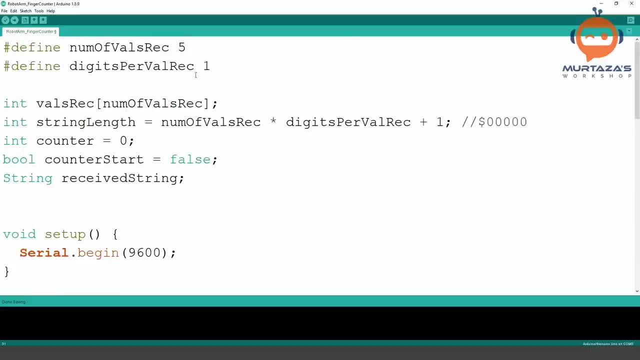 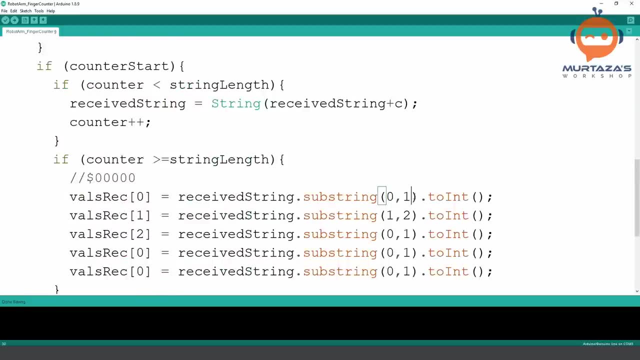 we will have one digit per value. so here we have one digit per value, but later on we might have two, we might have three. so again, we cannot hard code any values here. so we will use the digits per value here as well. so we can remove all of this and we can write here that four: 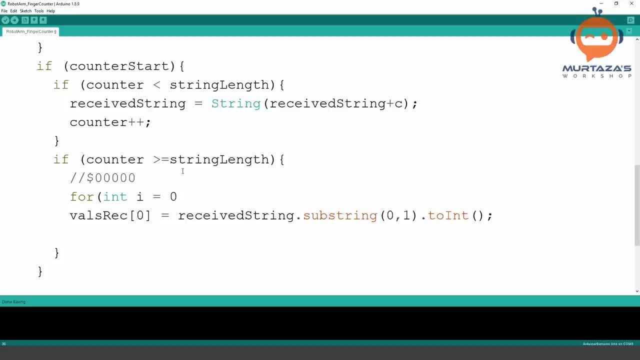 integer i is equals to zero, we are going to write: i is less than number, number of values received, and then we will do i plus plus. so while it is less than this value, keep adding to our loop, and then what we will do is we are going to create here a number. 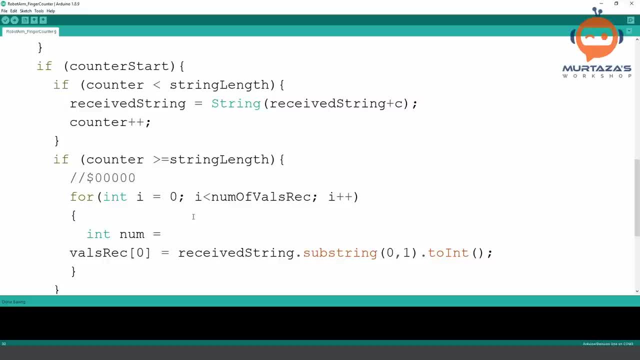 so we are going to call this: integer number is equals to i multiplied by digit per digits, per value received plus one. so this is basically our number. so the plus one is basically because we have our first digit as dollar, so we don't want to use that. 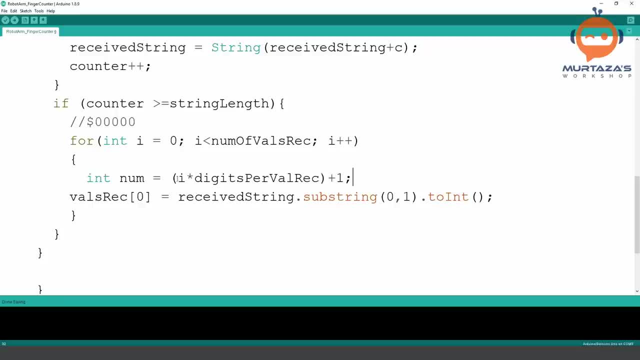 so we are writing plus one here. then we are multiplying the digits per value with i. so, for example, if we have the digit one, then it will multiply this with one. if we have digit 0, it will multiply it with 0. it will become 0. so in our first case, when it 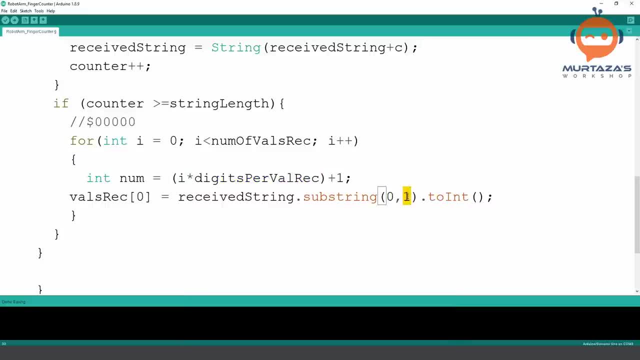 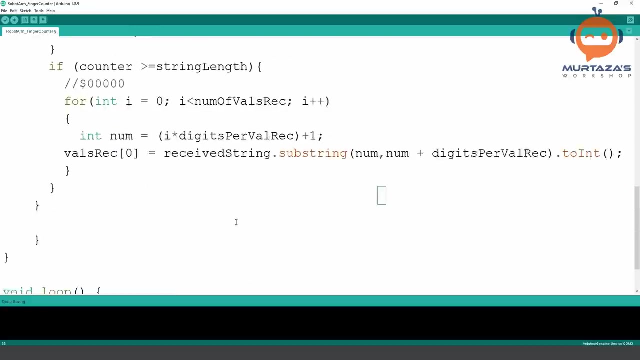 should be 0, this value should be 0, this value should be 1. right, so what can we do? so here we can simply write this number, number, and then we can write digits per value. we can write here number plus digits per value. okay, so this might be a little bit confusing. let me explain it. let me zoom. 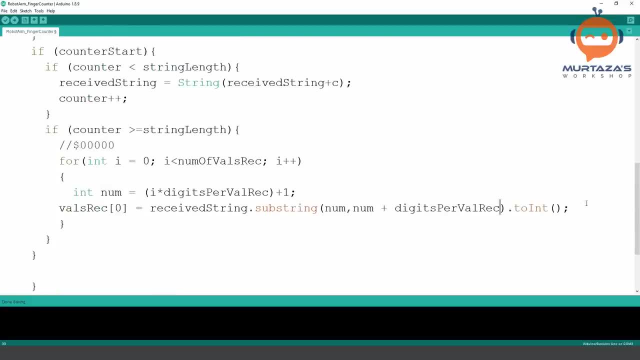 out a little bit. okay, let me explain what what's happening. so if I want my first, if I want my very first string, I will write here 1 & 2. if I want the second one, I will write here 2 & 3, because the first one is the the very. 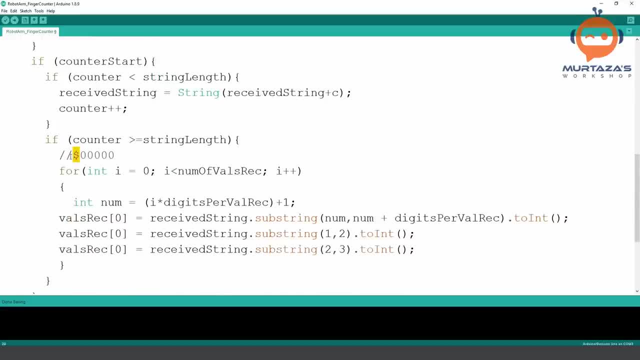 first one is the dollar. so actually I paste it here as well. so the very first one is the dollar. so we don't need that. so we are starting from 1 instead of 0. so we are saying 1, 2, 2. so this is basically the idea. so if we look at this equation, this will satisfy. 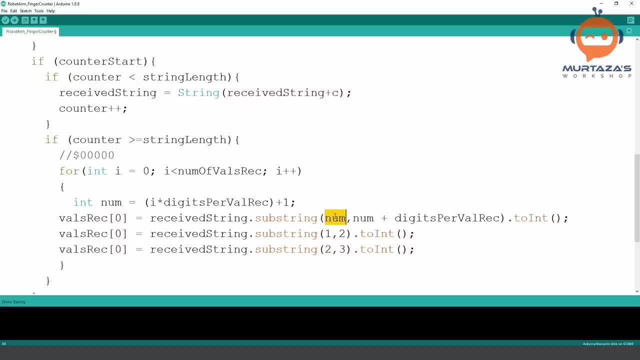 these conditions. so here you can see that we have number, so number here. if it is 0, then 0 multiplied by digits per value, it will be 0 plus 1, it will become 1. so this is 1. then the second one is: it's already 1 plus digits per value is: 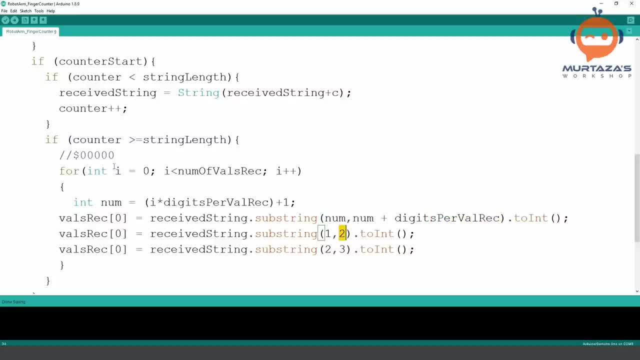 1, so it will become 2. then, if we go to the second iteration, this will become 1. so here this will be 1 multiplied by 1, which is 1 plus 1, so this will become 2. so here we are putting 2 and then 2 plus 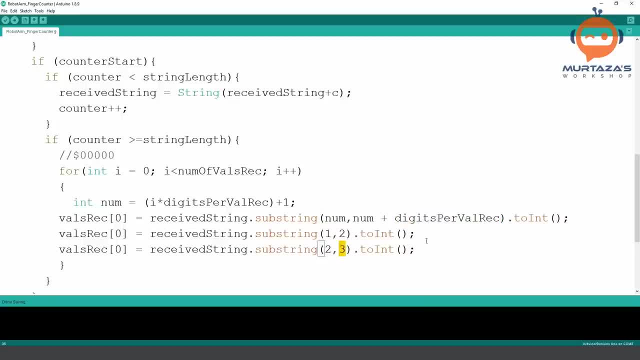 1, which is digits per value, becomes 3. now it is very easy to do plus 1 each time because in this particular case it is just digits per value is 1, but if we had more values for digits per value, then will become very easy to use. So this is why we have written it like this. I hope. 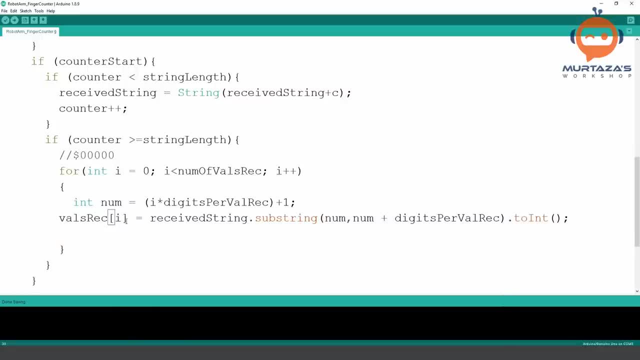 that was easy to understand, and then we can simply replace this with I. So hopefully we have not made any mistakes so far. So this will store all these values in our values received, and then we can use this value received for sending the commands to the servo. But then we need to refresh or reset our 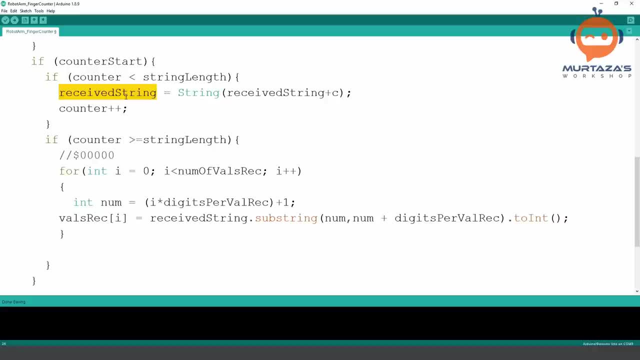 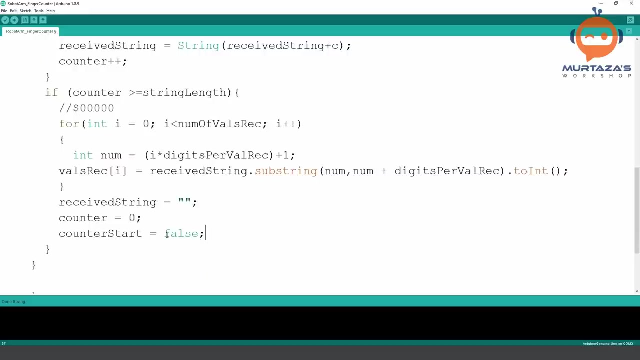 values for the second time it sends the string. So we need to write here that our received string is equals to empty, and then we are going to say counter is equals to zero and then we will say: counter what was it start? counter start is equals to false. So this will basically reset all the settings so that 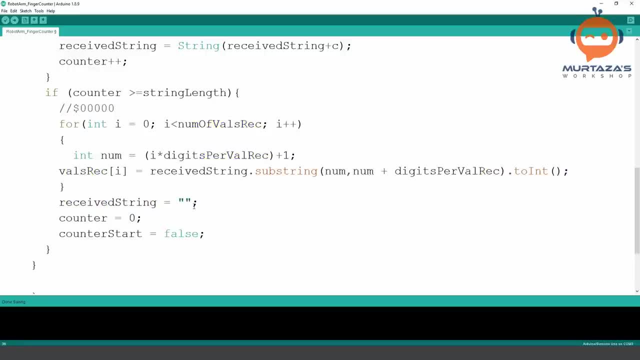 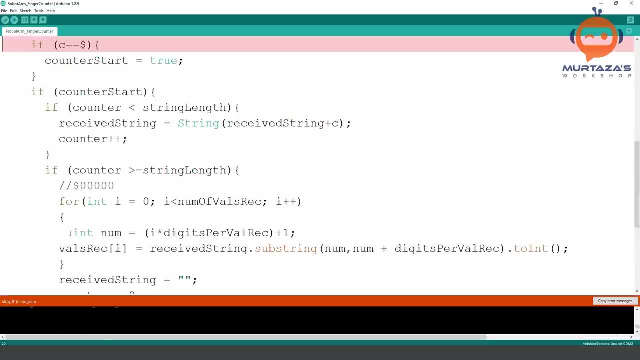 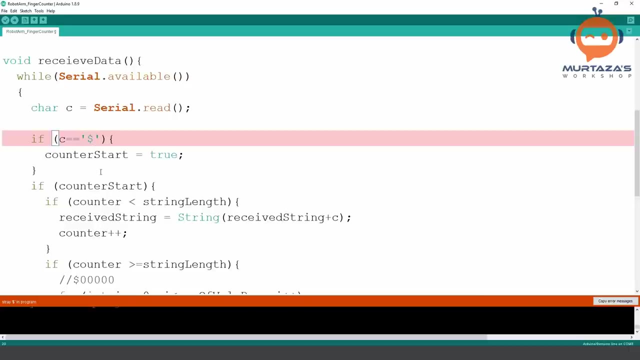 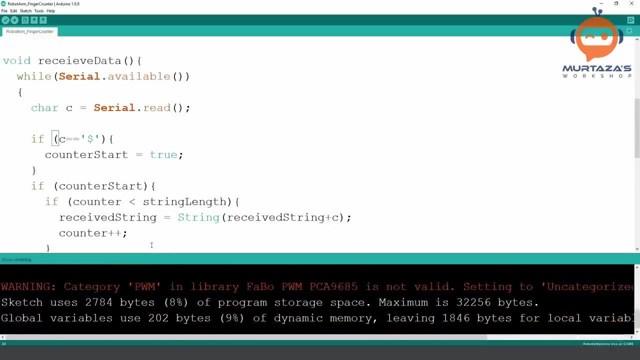 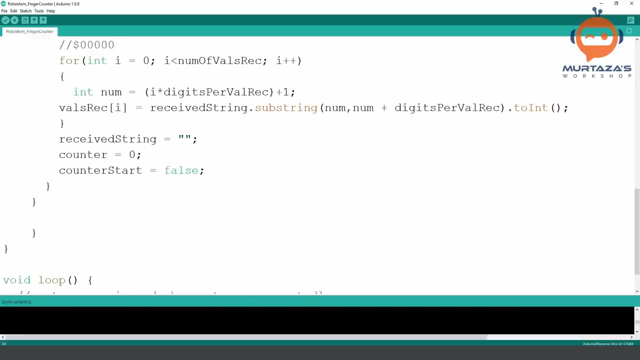 next time we can do all of this again. Okay, let's actually compile this, because probably there will be some mistakes. Okay, so C is equals to dollar. you have to put it like this: What else? Okay, so that was the only mistake, hopefully. Okay. so what else can we do Now? what we will do. 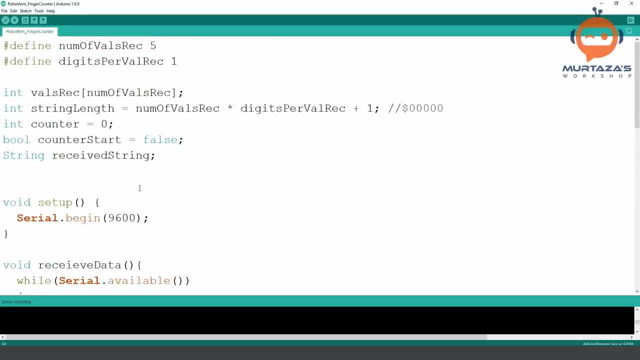 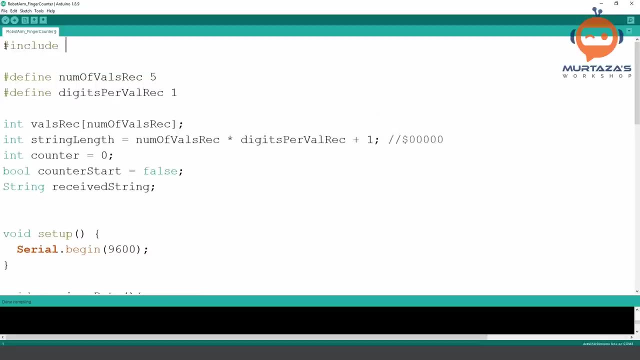 is, once we get to the end of the program, we are going to go back to our. we have to what do you call send it to the servo. So we will go up and we are going to write here that we want to include include servo dot edge and then 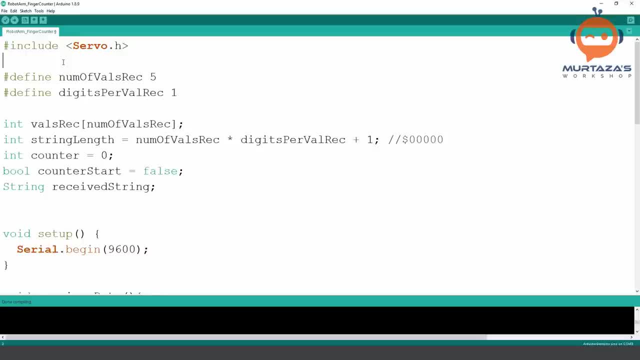 we are going to define or do we need anything else? Okay, we don't need anything else here. Then we are going to create objects. So basically we have our servo class and from this class we are creating objects. so each servo will have its own object. so we are going to write servo Thumb. Then 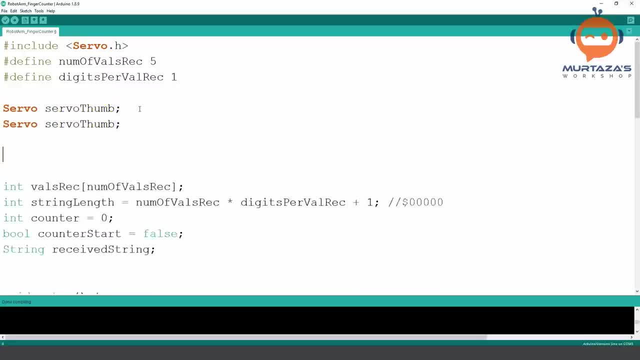 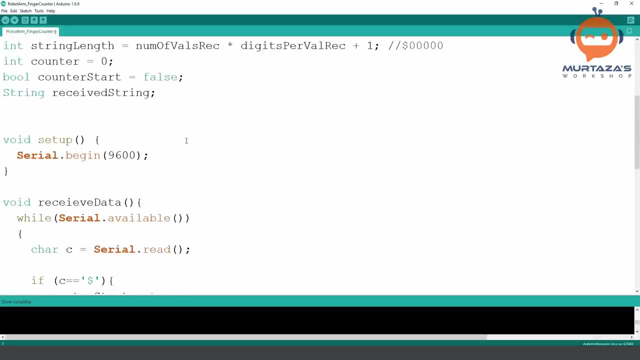 let's copy this because we are lazy. what happened there? Too many spaces? Okay, then here we are going to write thumb, and then index, and then middle, and then what is it? ring, then pinky. okay, so this is basically our initialization. then what do we need next? um, we need to define. 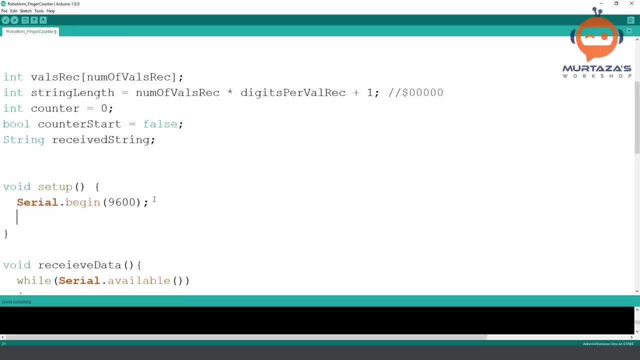 all of these in our void setup, so we need to define which pin number is connected to which motor. so what i have done, i have connected it in a very weird way. i just randomly connected it and then i tested each of these servos which one was connected right. 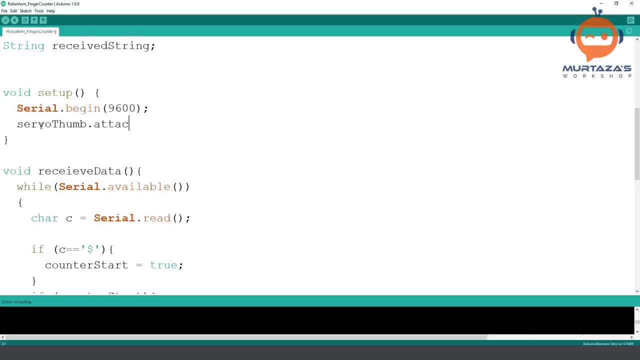 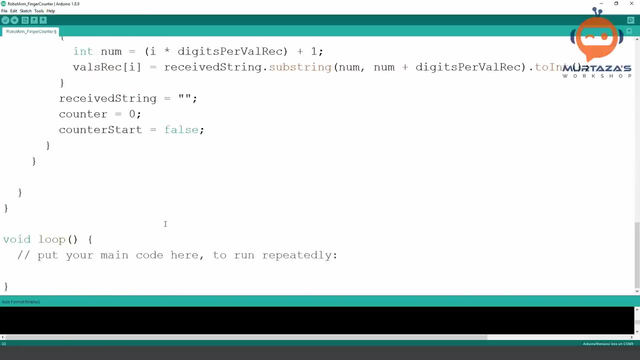 based on trial and error. so for the thumb we will write attach and it is attached to pin number seven. then we have: let's paste that again. it is paste open a little bit, let's not do that. there you go. actually, we can go to tools and auto format. 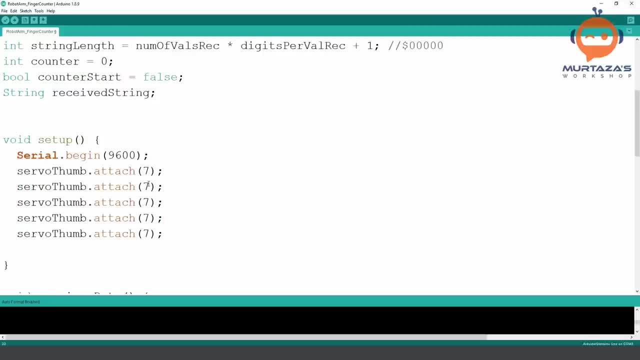 so we have anything we can add here. let's remove that. let's remove this here now. in this case, we backup it and there let's remove this. very只 that it looks very, very, very weird. let's remove that. yes, there you go. actually, we can go to tools and auto format that. 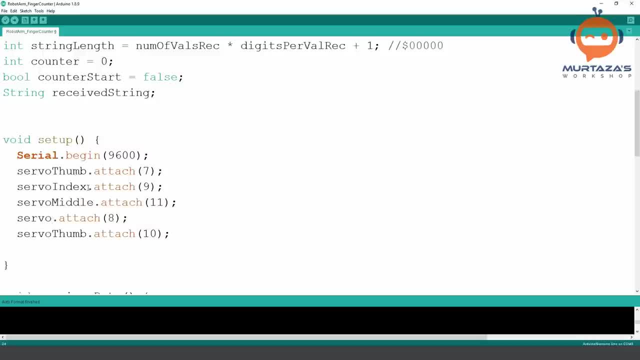 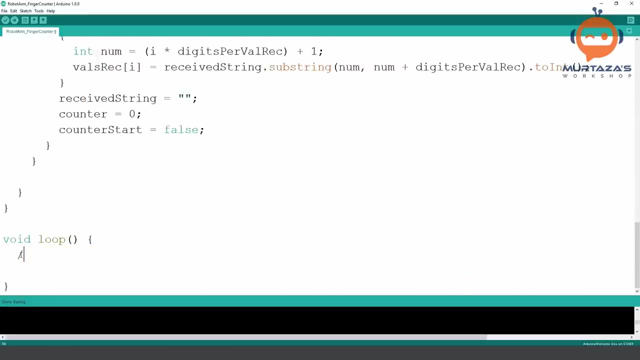 middle. then we have ring and we have pinky. okay, that is good. so let's save that and let's move on now. the, the last part is very, very easy. so all we have to do- if we, if we, did not make any mistakes- all we have to do is we have to first receive the data. 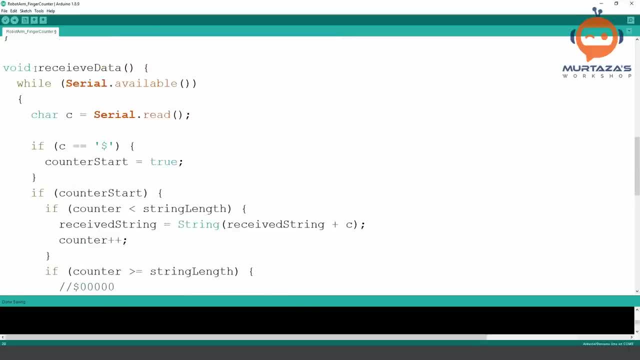 so we will write here. we will call our function receive data, and after we receive the data, we are going to send the commands to our motors. so we will write. if the values received at number zero is equals to one, so we will write if the values received at number zero is equals to one. 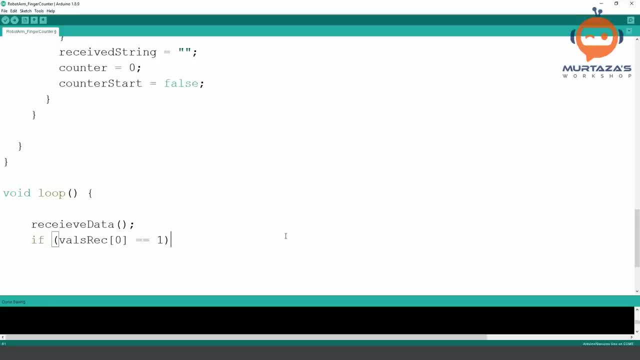 which means open it up. then we will write servo thumb dot write. we are going to send the command as 180, so we will rotate in one direction. else else we are going to write servo thumb dot write zero. i'm writing it in one line because it's 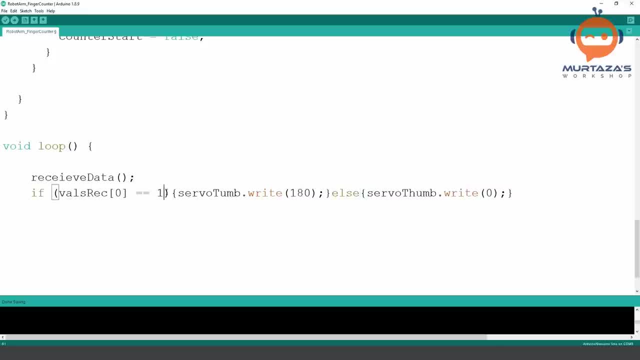 easier to read that way. so we are going to write servo thumb dot, write zero. that way, you will see now, uh, we can just simply copy this and we can paste it multiple times, and yeah, so that makes it very easy to read what is happening. you could write it in separate lines. 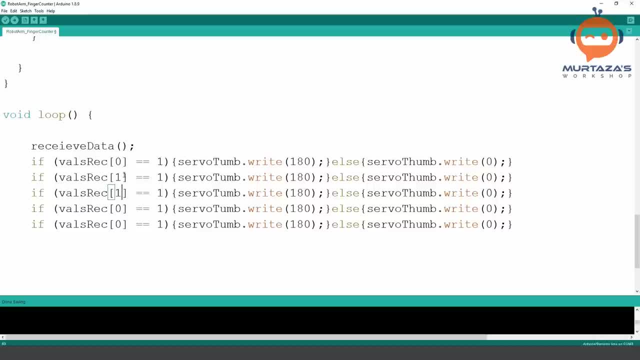 as well. so here i can just replace this with one, two, three and four, and then we need to replace these with our other values. so we will write here index. i should be capital. then we are going to write here index. and then we will write here: middle, servo, middle, we'll write. 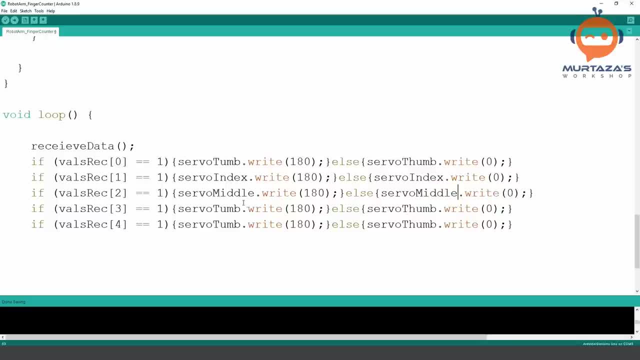 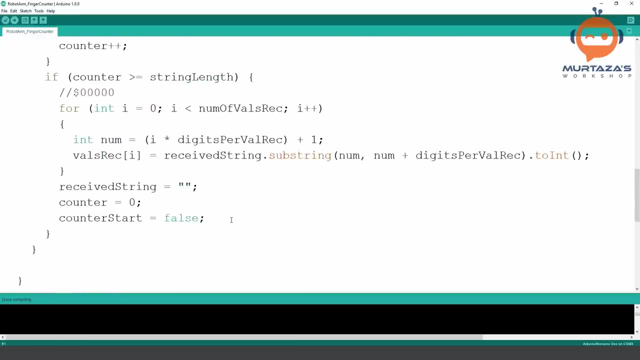 here, middle ring, ring and then pinky. okay, so that actually looks good to me. let's compile and see if we made any mistakes. of course, thumb, what else? oh, it's working. that's great, so hopefully it will work now. so, before we go ahead and start the actual test, so we are going to go ahead and start the actual test. 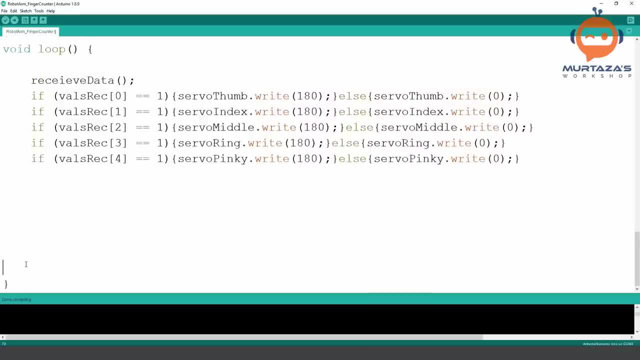 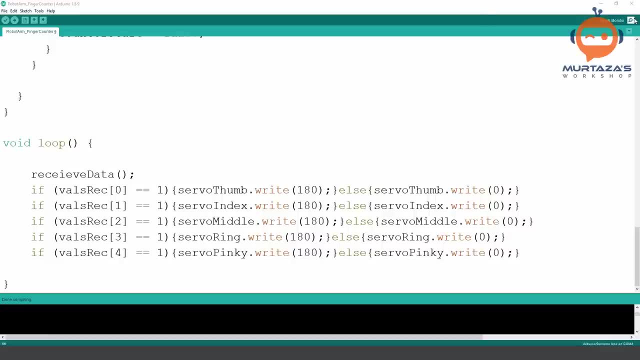 okay, so we are going to go ahead and start the actual test. so we are going to go ahead and start the actual test. we go into our what do you call a Python script? we are going to test it here. so how can you test it here? basically, you can open the serial monitor up and as. 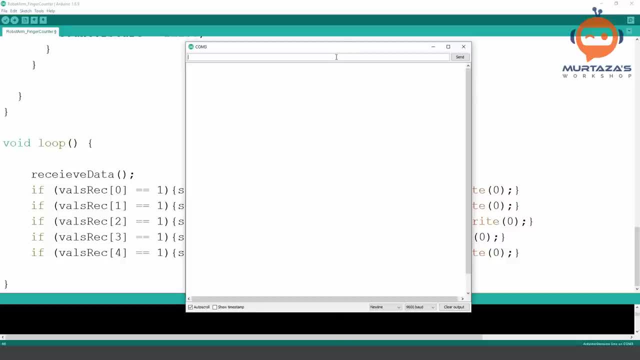 you can see, you can hear the voice already. what you can do is you can write here the signal and then you can send this command and see if it works. so what I'm going to do is I'm going to record the hand and record this at the same. 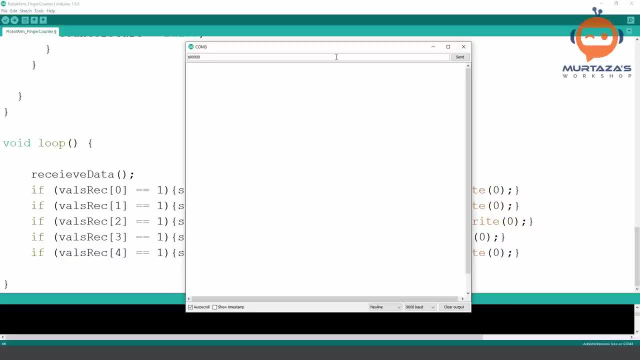 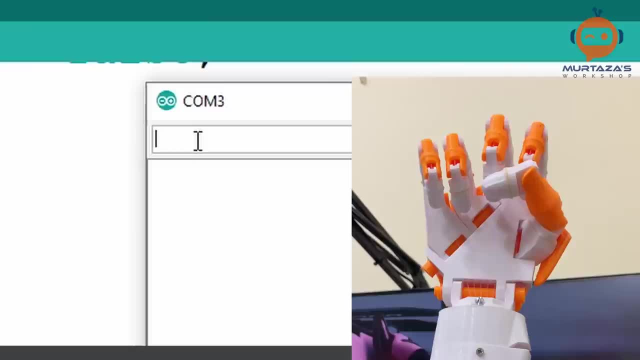 time so you can see how exactly does it behave. so let's try this out. I'm going to add zero for all of them and see if anything happens. so nothing so far. then we are going to write dollar, then we will put all of them on. so we'll put five. 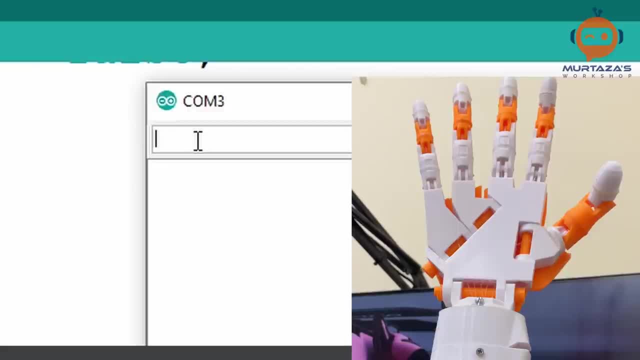 ones, and there you go. so all of them open up, and then we are going to try one of them to close. so what we will do is: you can see that it's not working, so we are going to try to close it, and then we are going to try one of them to close. so what we will do is: 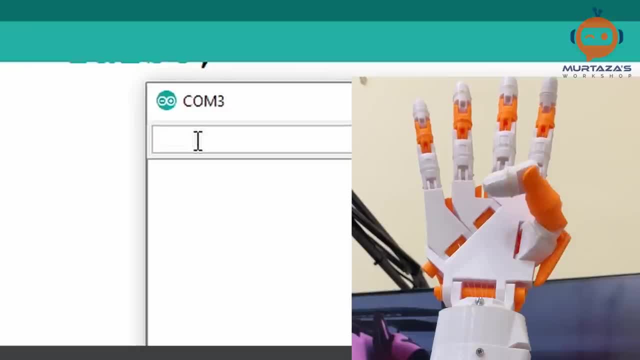 we will put zero, one, one, one one. so there you go. then we can put. we can put, let's say, one, zero, one, one one. there you go. so now you can see that when I send a command it actually behaves as we expect it to. so there you go. so all of them off. 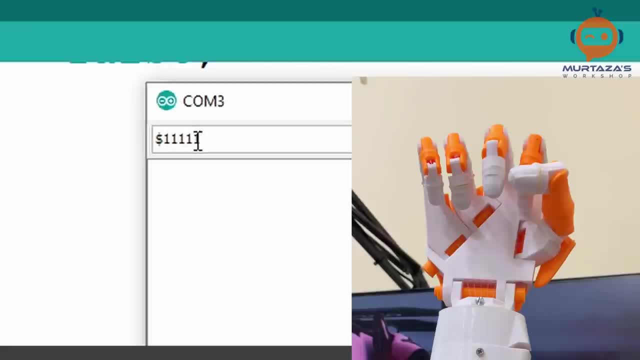 and then we can send all of them to the next one. so this is the command that we are going to do on. So this is basically the idea. Now, What we can do is we can go on to our Python script and we can Send this string from Python instead of writing it manually. 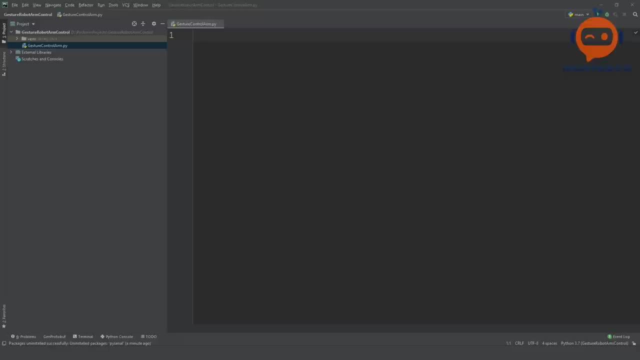 So here we are in our PyChamp project, and what we will do is we will create the code to actually send the command To our Arduino board. now the commands will be sent based on the gesture part. So we will also look at hand gestures, So we will look at how many fingers are up at any given point and based on that, we will send the commands to the Arduino. 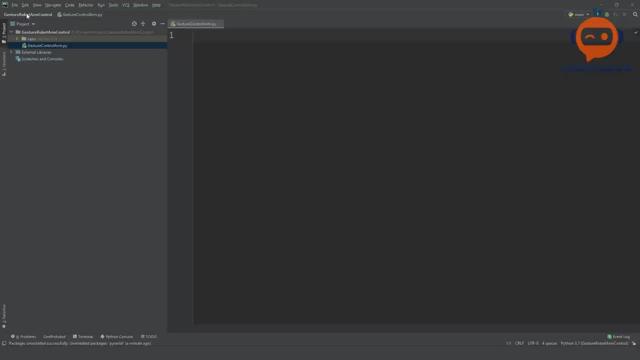 board. So what we can do is we will be using media pipe liability to actually track the gestures. but the thing is that we have created a module out of this and We have packaged it together in one simple- What do you call it? package, and you can install that. 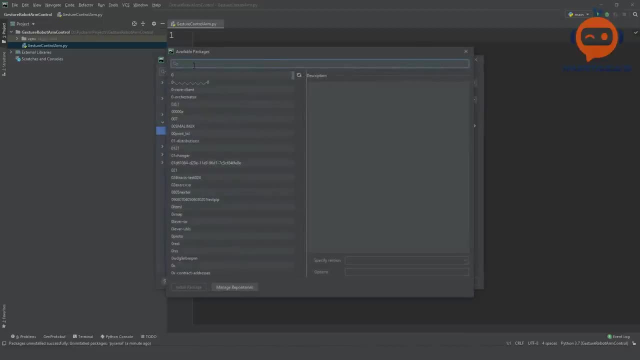 By going to the project and you can add, and here you can write CV zone and you can simply install this. So this includes the serial communication part as well, and it also includes The hand tracking part. So all we have to do is we have to call these methods and 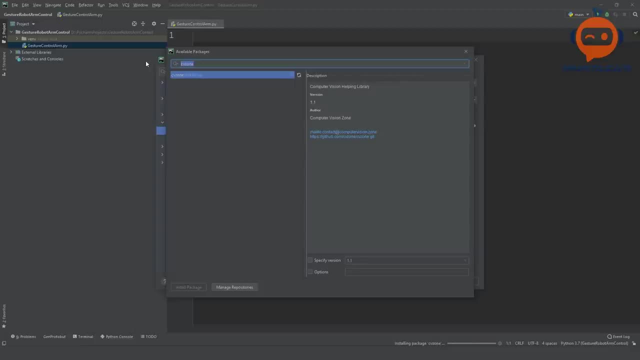 Then we can make use of them, and this will install The open CV and the media pipe library by default, but it will not install the serial part. So what we have to do is we have to search for serial Now. the serial by default did not work for me, So I tried serial device and that worked fine. 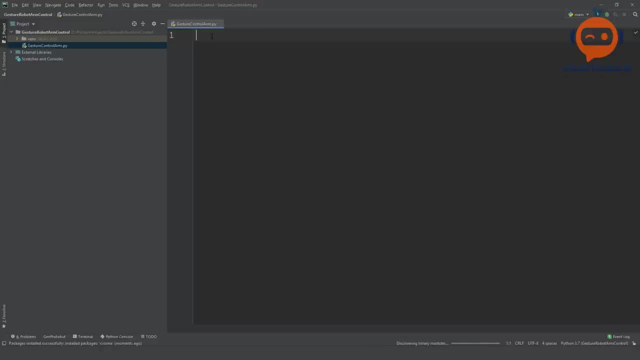 So now both the packages have been installed and you can see that we are in a python file called gesture control. So we are going to import here CV zone and then we will import CV 2. Then we will write: cap is equals to CV 2 dot video capture. 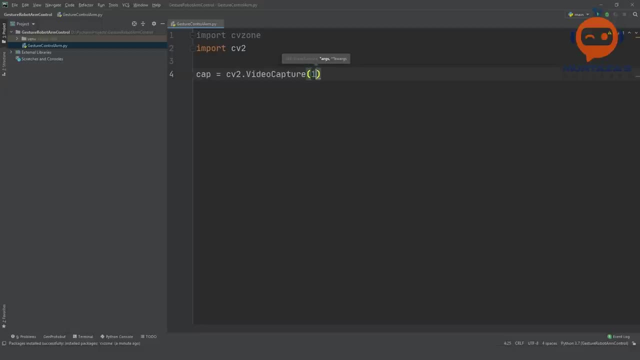 And we are going to say that our ID number is 1, so you will probably use 0, and then we will write cap dot sets and We are going to set it, or do we need? we can skip this if we don't want to give it any size by default. 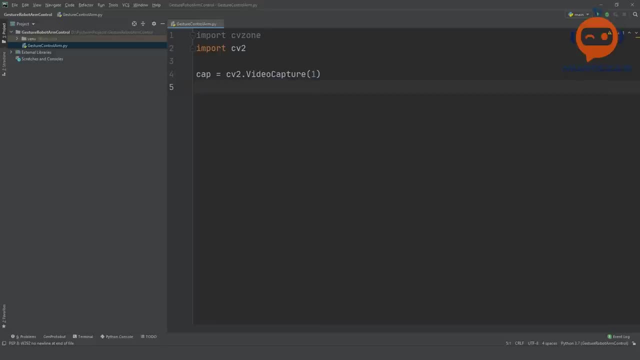 The camera I'm using is 640 by 480. So that should be fine. then we need to Write the while loop. So while true, We are going to say the success and the image is equals to cap dot read. so this will read the frame and 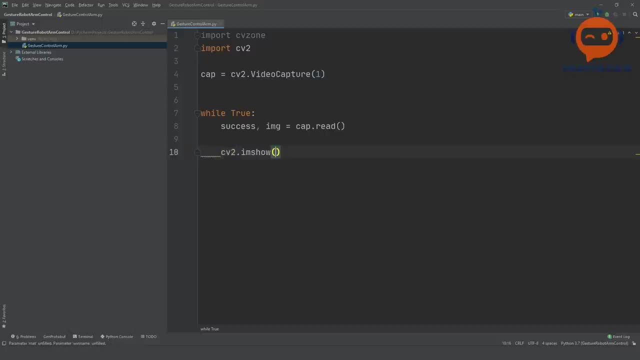 Then we will simply write: CV 2 dot. I am show, and we are going to show the image, a image, and then we will say: I am G, and what else? cv2 dot, wait key, Wait key, and we will put one. so this should run Smoothly. let's try it out. 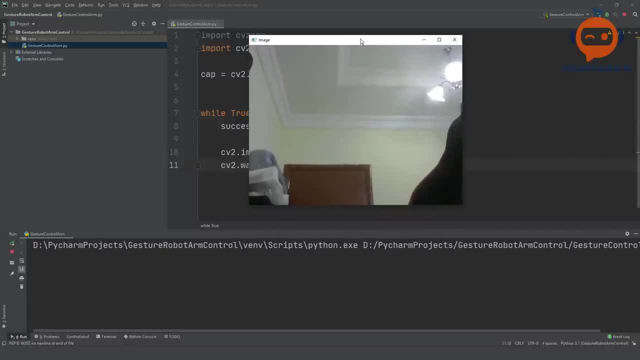 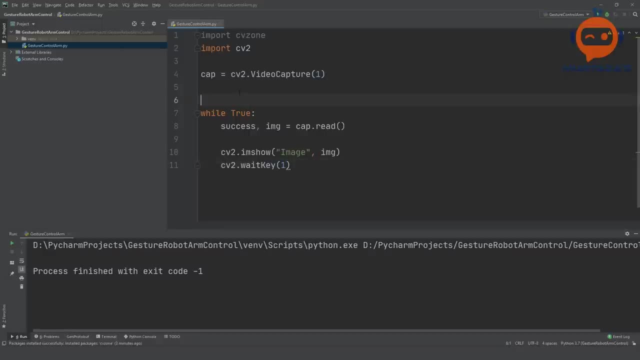 There you go. so, as you can see, here is my hand and you can see that it is working fine. So now we will add the hand tracking part, so this functionality is Provided by media pipe library. now media pipe library is already installed, because we installed CV zone and 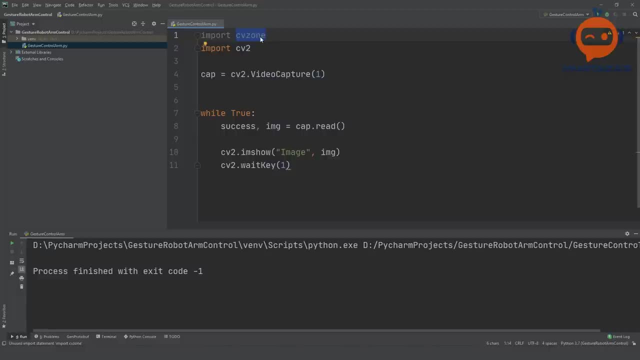 Within CV zone we have a module that makes it easier for us to get the values from the media pipe library, So it's like a wrapper. So here we can write: the detector is equals to CV zone dots hand detector and if you want, you can give in some parameters and 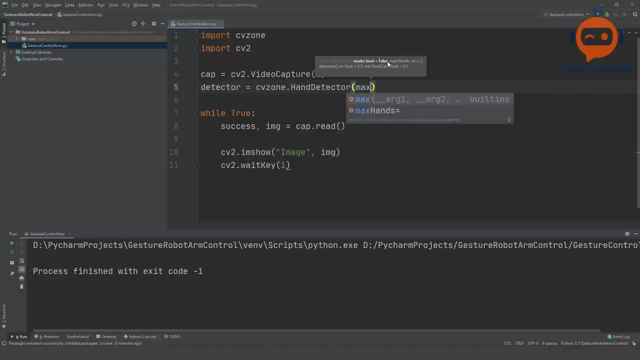 like the maximum number of hands. so actually we should give the maximum number of hands as one and the detection value you can decide. the detection confidence can be anything. by default it's 0.5. so then we are going to find our hands and we can simply use this object that we just 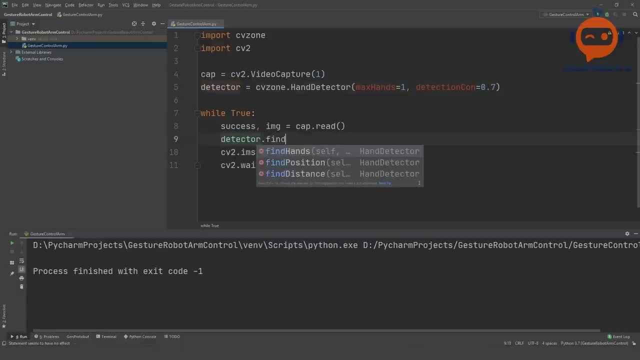 created. we can write here: detector dot- find hands and we will give in our image and it will return us with the image, with the output drawn, so we can grab that. then we are going to find the position of our hand. by position we mean the landmarks. so we will write here: detector dot- find positions. 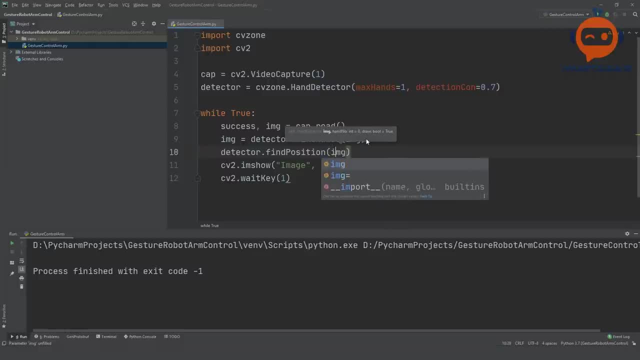 and then we are going to give in our image and we'll will also take in return. we will take the lm list and we will also take the bounding box. so that should give us some detail, and then again we can print this out. so let's try it. 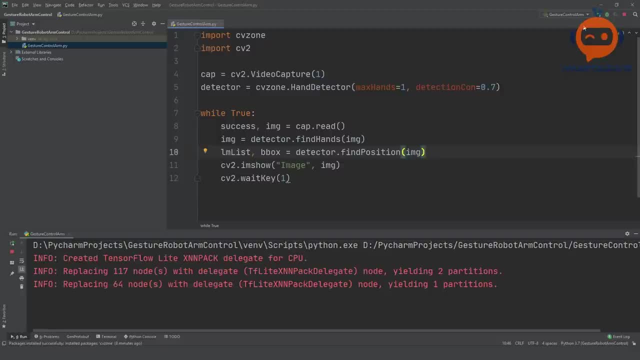 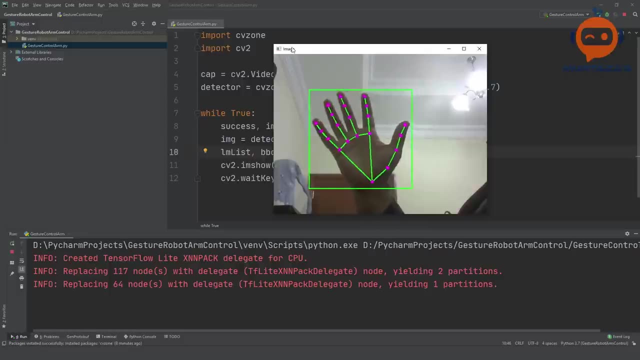 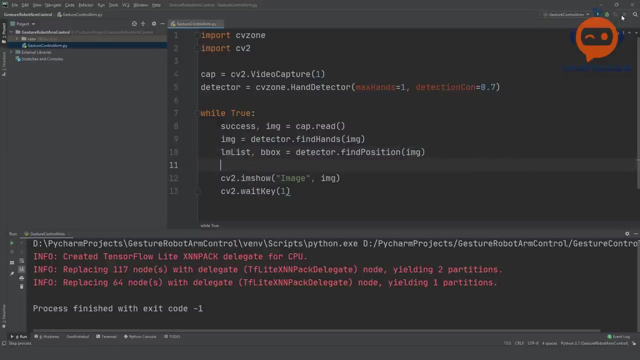 so here is the image, and if i put my hand in, you can see that we have some tracking and we can see that we also have the bounding box. next we are going to check how many fingers are up, and again, this is very easy with our package. so 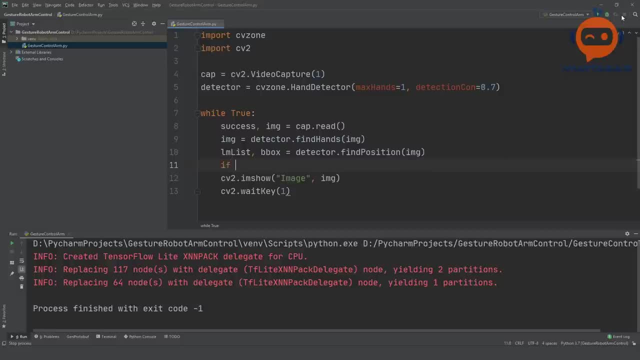 we can simply write if lm list. so if lm is left, you'll just simply net this function. there is something available. then we are going to say that detector dot fingers up. this will tell us how many fingers are up and we can simply write here fingers so that we store it in the list: fingers. so let's print this out, we will. 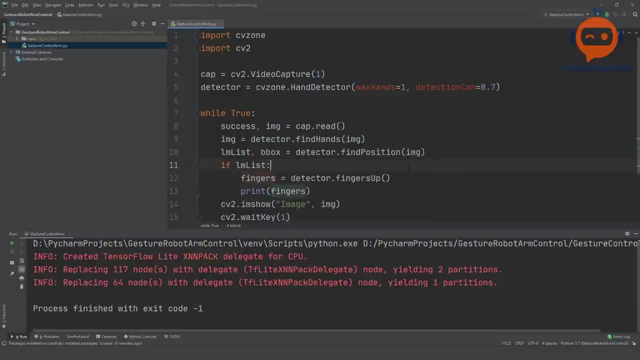 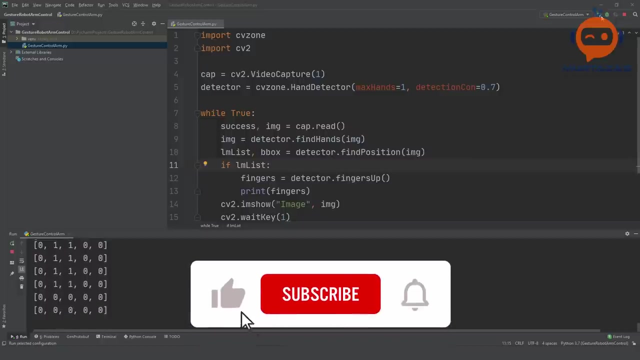 write here fingers, there you go. so let's run that. so right now you can see, all of the fingers are up and if I put all of them down you get zero. then one, two, three, four and five, so all of them are working fine. so- and this the best part here- is that this is the exact same format. 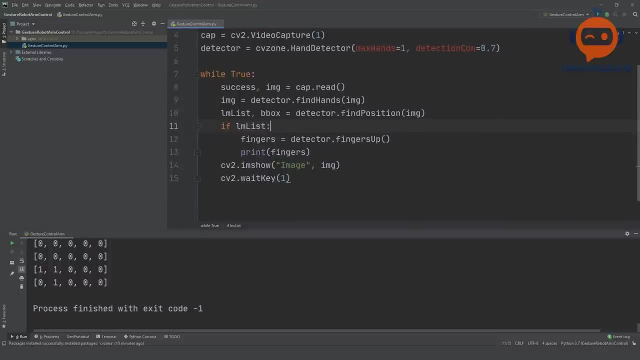 that we used in Arduino. So all we have to do is we have to send this fingers list to our Arduino, and that should work by default seamlessly. So how can we do that? To do this, we have the serial module within the CV zone package. 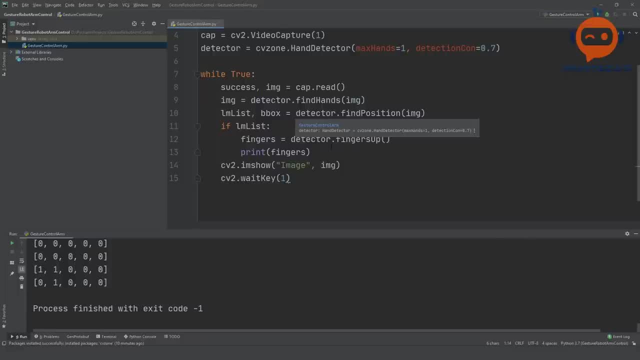 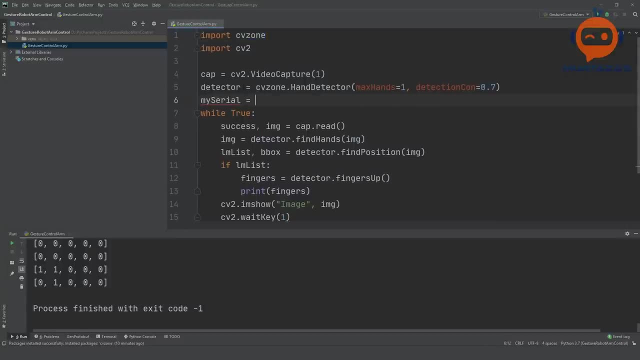 So it allows us to communicate with Arduino. So, in order to use this, the first thing we will do is to create a serial object. We will call it my serial and we will write here that CVZoneSerialObject. And now we have to give in the configurations. 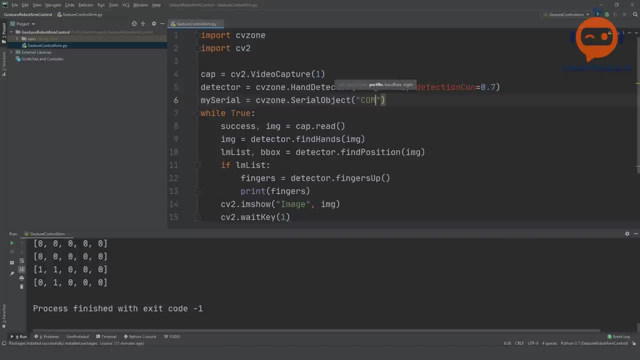 So, as we saw earlier, we are using COM3, the port number, and then we have to give in the baud rate. We select it as 9600. And then we have to decide how many digits are we sending per value. So in our case, we are only sending one and zero. 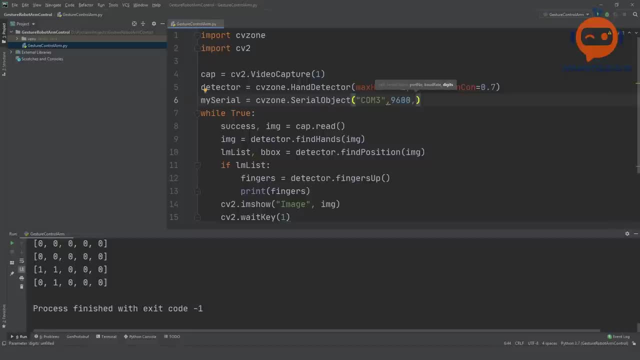 So it needs only one digit to tell whether it's working or not. So we will write here one. So if you're doing something else, you have another project. definitely you will have to check how many values you're sending And based on that you can change this value. 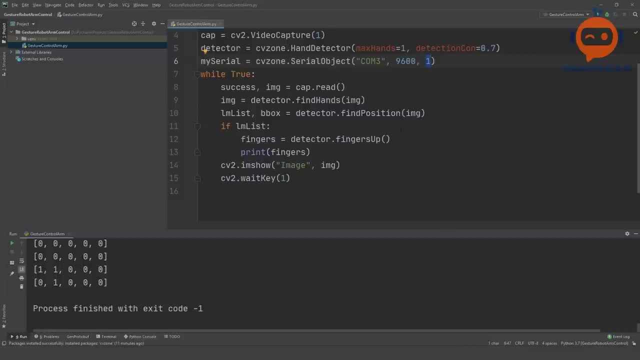 So once we declare this, now all we have to do is we have to send the data. So we will write here mySerialSendData, And here we are going to send our data. Now. this is the easiest part, where we just write fingers. 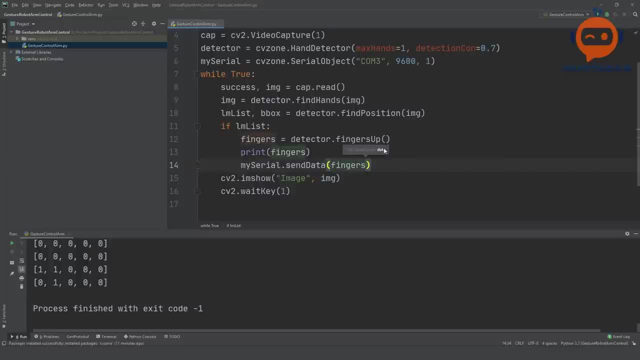 and it just goes to the serial And it should work by default. So all we are doing is we are getting the values from our detector and we are simply inputting it to our send data for our serial object And let's see if it works.